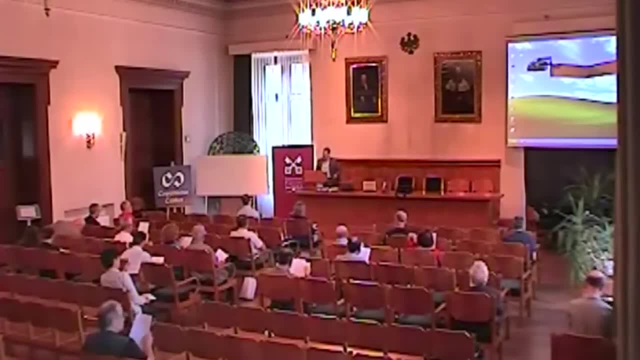 word that I, a practicing card-carrying intuitionist, just uttered, as well as every word uttered by my conventionalistic or classical colleague, Professor Abramson Further. I wager that, on the basis of that common or shared understanding, you came to know at least that what I said. 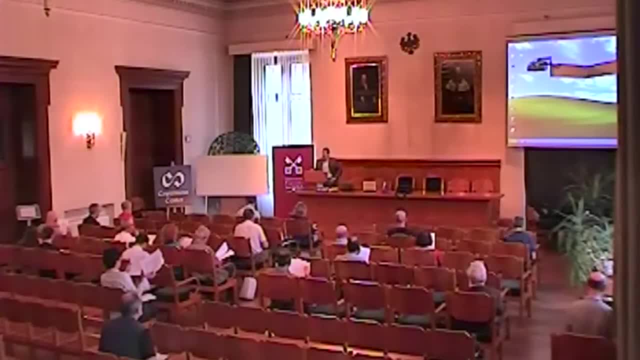 enunciated some plain truths of intuitionistic mathematics. Thank you. I am not concerned to sort out the various truths from the various falsehoods, to determine which of us, if any, is right and which is wrong in those assertions. Rather, I wish 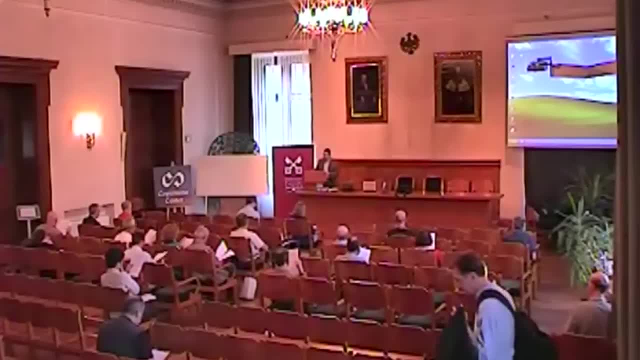 to concentrate on a fact that I take to be obvious and unassailable, namely that my assertions in each pair contradict the corresponding truth. Thank you, I am not concerned to sort out the various truths. Rather, I wish to concentrate on a. 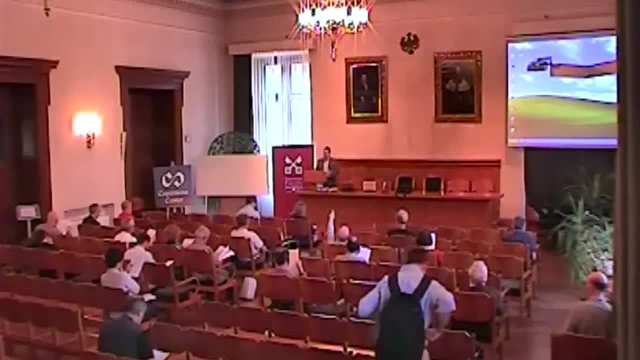 fact that I take to be obvious and unassailable. I am not concerned to sort out the corresponding truth. Rather, I wish to concentrate on a fact that I take to be obvious and unassailable, The corresponding assertions of my noble and illustrious colleague. that is, that when 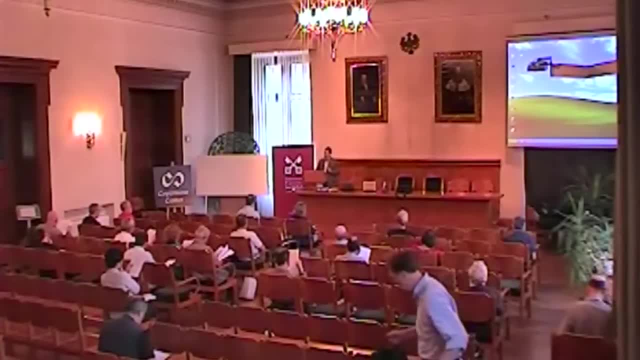 he spoke and I answered. what I said contradicted what he said And what could be. One question: When you say it is false, you say it is false then, was it? it is false because the card-carrying intuitionist is a believer in understanding. 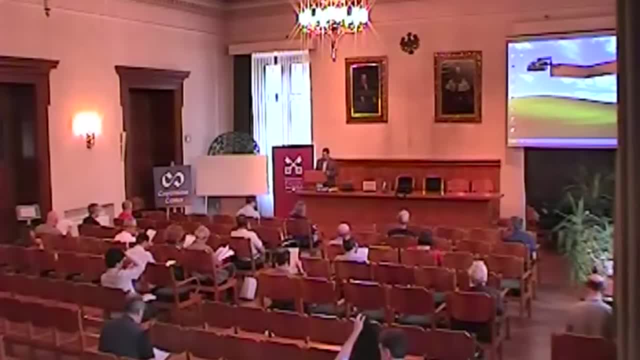 I shall answer that question. And what could be plainer than that? After all, much of what is properly called the correct expression is the correct expression of the card-carrying intuitionist, of the critical bearing of intuitionistic mathematics would be lost altogether if we intuitionists refused. 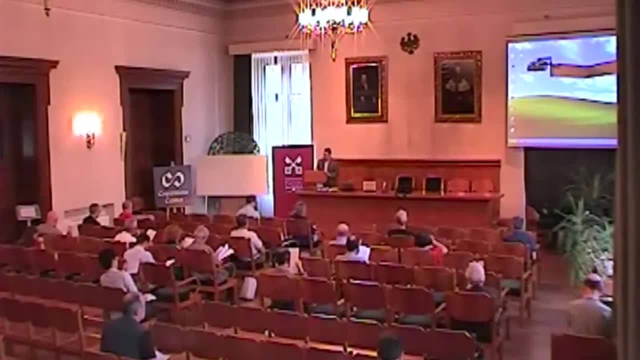 the liberty to decry and deny such falsehoods as the general law of the excluded third, the tertium non doctor, to take one example perhaps overly prominent Today, I hope to prove right before your very eyes that the acceptance of a general mathematical realism 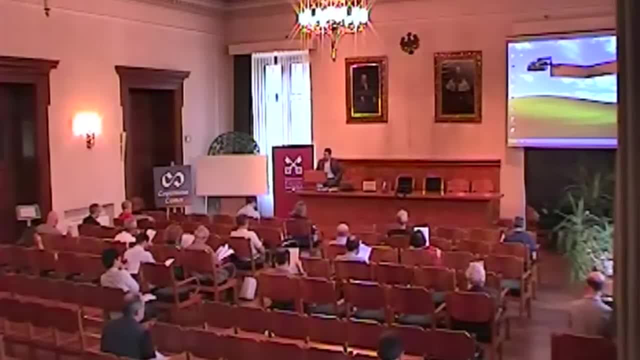 even in a mild form, convicts one of the existence and reality of outright contradictions in mathematics, As befits a conference with this title: Church's Thesis. Church's Thesis will play a prominent role in that, As usual, despite old Hilbert's repeated insistence. 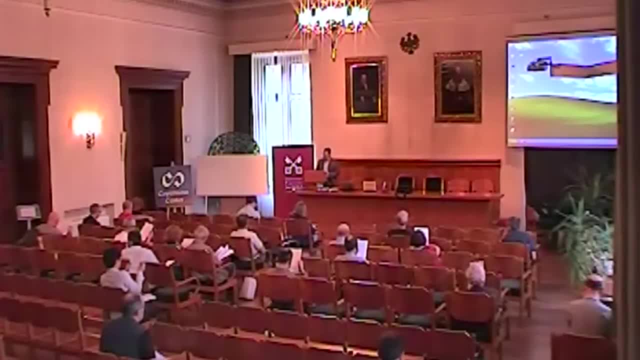 to the contrary. there is more than a little trouble now in Cantor's Paradise. I hate to point it out, but in Cantor's Paradise, as in more terrestrial climes, property values lately stand at disastrously low levels, Apart from yours truly and a small number. 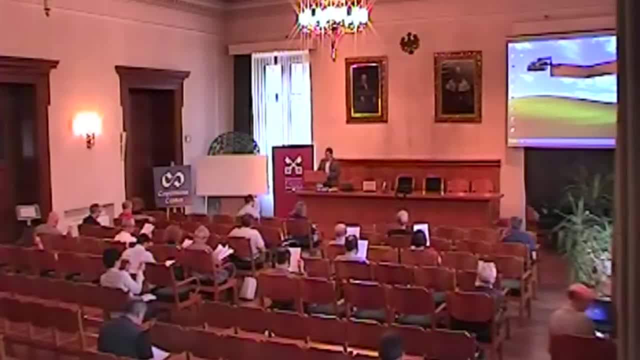 of right-minded disciples. every philosopher of mathematics, Stu that I know would want to deny vehemently, utterly and comprehensively my insistence that any conventional statement or classical statement from the first group, page three, as uttered by my colleague Darren, 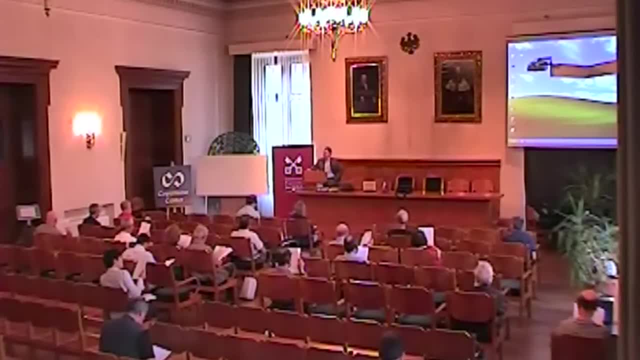 contradicts any statement of the second group uttered with all due seriousness by yours truly. Now, and I have to ask this even though it is sad and embarrassing- what would lead one to endorse such a preposterous doctrine? In answer, one can, I think, point out a number of in. 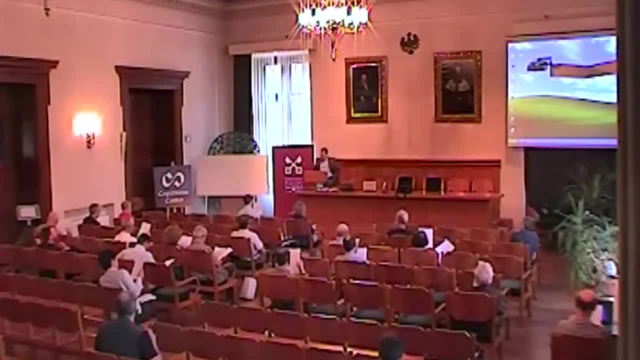 any way realistic, logical and logical influences. One hesitates to call them reasons, some of which are historical and others theoretical. I shall restrict my treatment today to one of the more salient of historical influences, As is so often the case in this veil of tears. 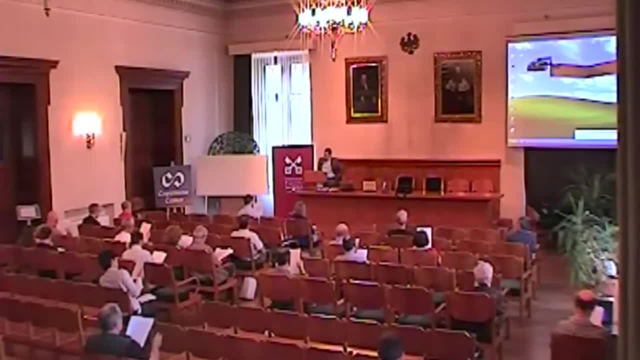 the historical influence I have in mind is a glorious hangover, a humdinger of a hangover. It's a hangover from a binge drunk and an idea once occurrent among the logical positivists of yore. principles of mathematics, all of mathematics, intuitionistic as well as conventional, are 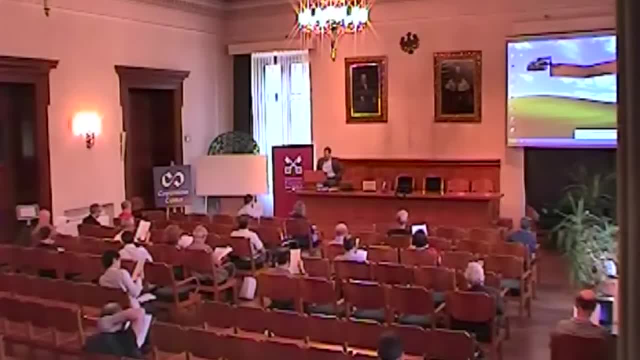 number one, true, and number two owe their truth entirely to the meanings of the various linguistic terms that feature in them. In order to shore this up their positivistic fantasy about meaning, the positivists had to play fast and loose with meaning and demand, in the face of obvious contradiction, that 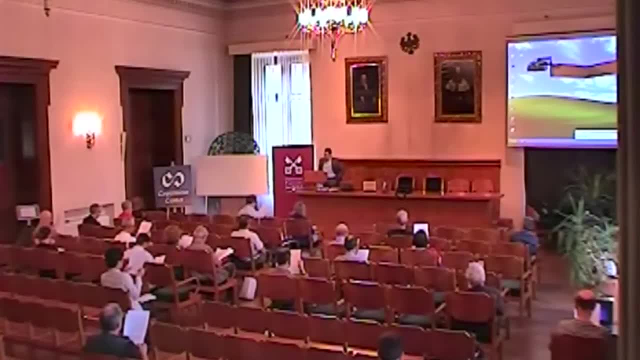 the terms featuring in the statements of the intuitionists do not possess the plain, ordinary mathematical meanings that they so clearly possess. Furthermore, the positivist insisted that those selfsame intuitionistic meanings, once exposed, must be seen more or less immediately to certify the main claims of the intuitionists. 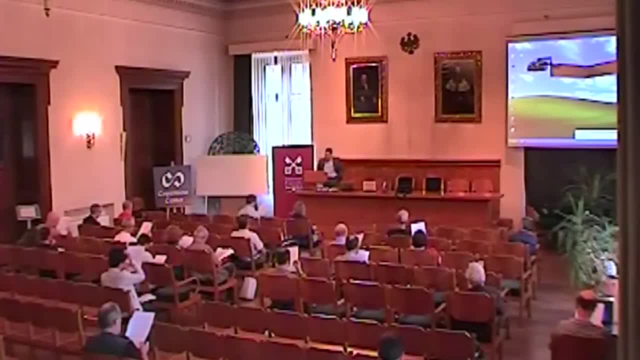 as true. I remark en passant that this was not a burden that many were seriously eager to impose equally upon conventional mathematicians. Few scholars, then or now, insist, They insist that the axiom of regularity, for example, be an immediate expression of. 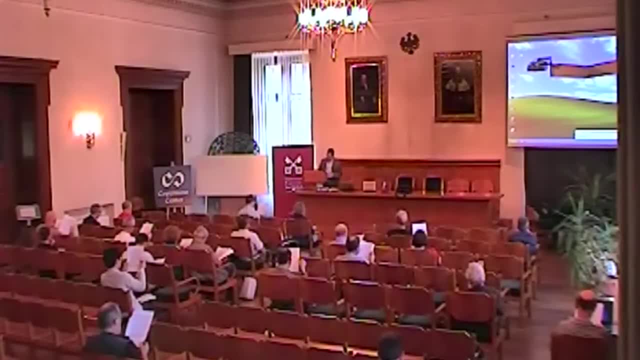 the meanings of such terms as set and member. I will not have the opportunity here and now to perform the complete demolition on this silliness page four, that I would so much like to perform At the moment. however, suffice it to say that, try as they might the logical positivists 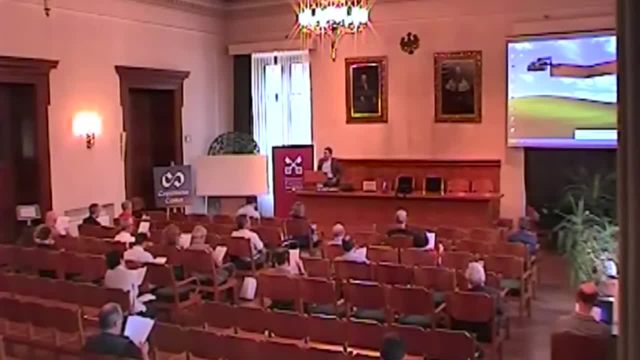 of then and their fellow travelers even in the present day could never come to any firm agreement on what those strange, antinomial, intuitionistic, mathematical meanings of the present day were. Let me run through a few of their lamer suggestions. 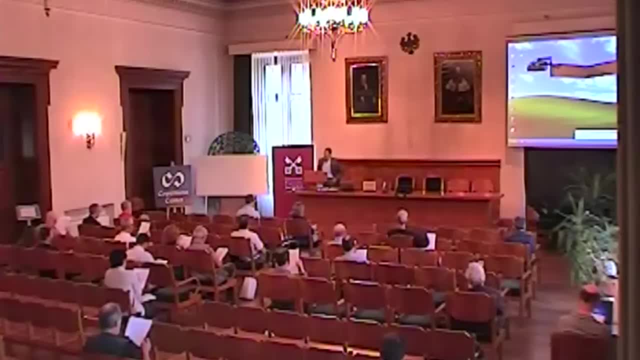 Number one. first, there are those who once believed that the main culprit and bearer of a specifically intuitionistic meaning is a logical sign, the humble and innocent existential quantifier, also known as the backwards E. The idea was that the intuitionists are supposed to attach a special constructive meaning to 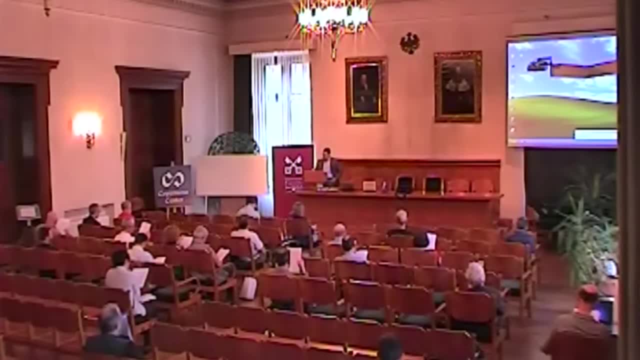 the existential quantifier that is not attached to the same quantifier when it appears in conventional mathematics. In response to that suggestion, I point out that the logical rules for quantifiers that the intuitionist Aaron Haitink once codified, the rules of formal intuitionistic logic for 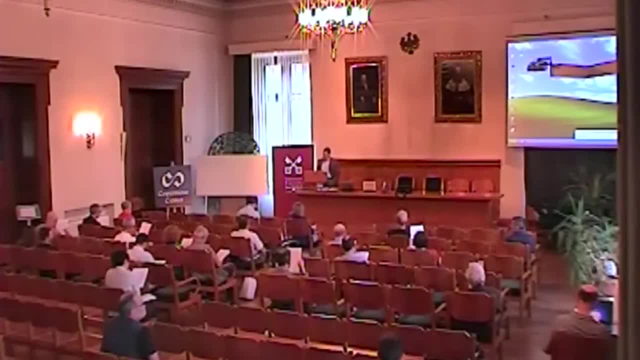 the quantifiers do not in themselves differ one iota from the familiar formal rules of the quantifiers in conventional logic. Those rules, folks, are the same. Moreover, as is well known, forms of intuitionistic set theory agree with conventional set theory. 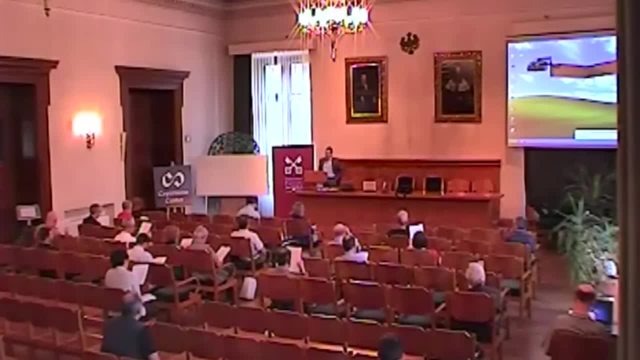 up through pi-0-2 statements over the natural numbers, that is, universal existential statements on the natural numbers. Moreover, conventional and intuitionistic mathematics do not, in general, agree when it comes to theorems that do not contain the backwards E. 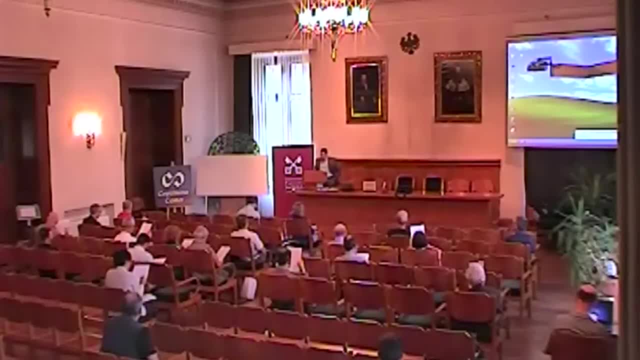 For example- and this will play an important role in what is to come- the negated form of the halting predicate or, if you prefer, the non-halting predicate, that is, there's no number m on which Turing machine index n halts. this provides a counter instance to 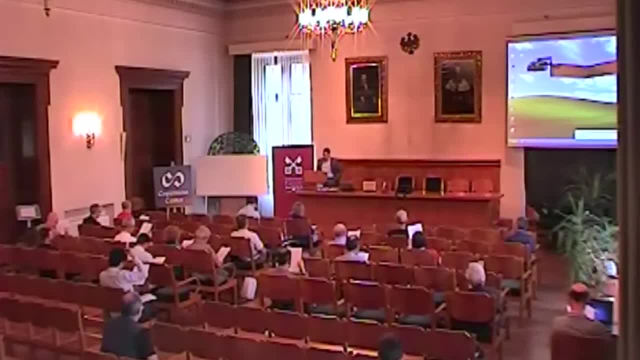 the Tertian non-dator. This is provable in intuitionistic arithmetic And this theorem can be formulated. It can be solved perfectly without any appearance of the backwards E. Lastly, there are any number of appearances of the existential quantifier in expressions. 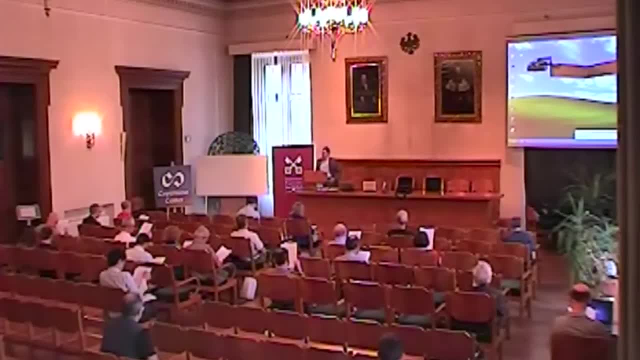 of truths, of intuitionism that cannot reasonably bear a constructive interpretation. There are finite- excuse me, there are transfinite. there are finite ones too, but there are transfinite cardinal numbers. There are lawless sequences, that is, sequences that are absolutely non-rule governed. 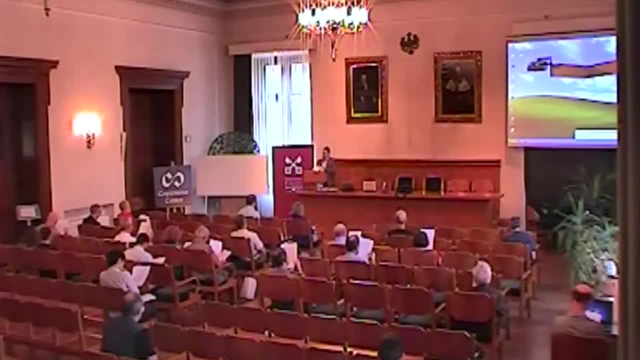 And every set has a power. set are three of those truths. I choose them at random. Page five, Second suggestion On this next tale of meaning change: negation is the culprit. It's thought that the sign for negation is to bear some peculiar or special non-standard. 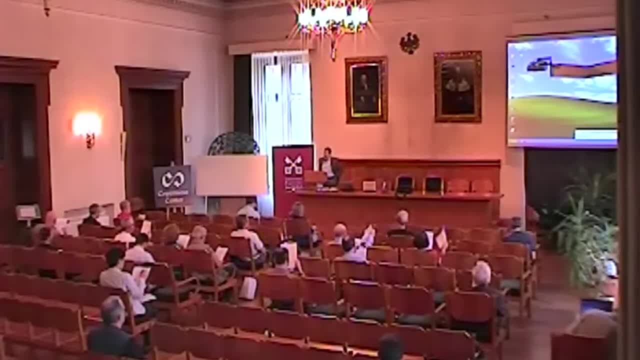 meaning, a meaning that perhaps makes it a stronger negation than its conventional brother. The trouble with this suggestion is that advocates of the non-standard negation view could never come to a generally agreed formulation of what that special meaning is. Furthermore, from the supposition that there is a specifically intuitionistic, then there's 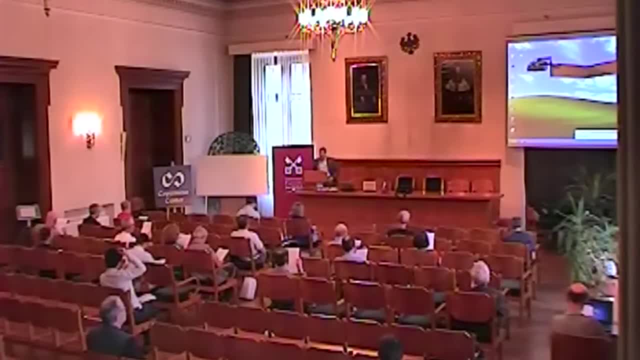 a two-way reaction. That's one thing, negation, and that it accounts for the differences between intuitionistic and classical mathematics. we get no explanation whatsoever for the differences that do not involve negation, For example the fact that Peirce's law- there it is, if P, then Q, all, then P, then P is not a theorem. 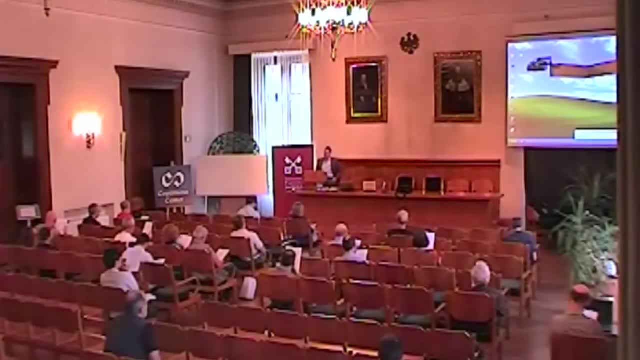 of formal intuitionistic logic. That's one of them. right, This is the theorem of conventional propositional logic, but not of intuitionistic formal logic. The fact that every total natural number valued function of the natural numbers is recursive is another such fact. 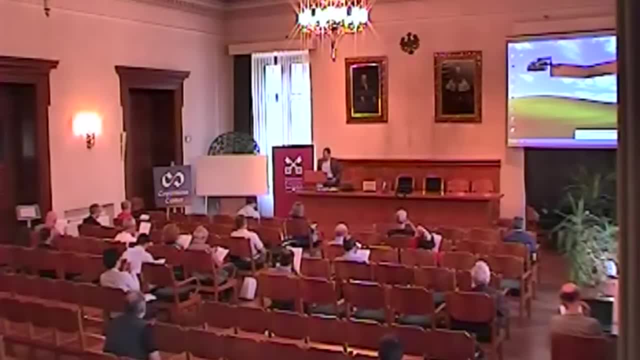 Third, there are those anti-realists, acolytes to the beatified Michael Dummett, who preach that all the logical connectives and quantifiers of intuitionism are at fault, not any one in particular. They are all supposed to collaborate in pulling a semantical trick, Making my words. 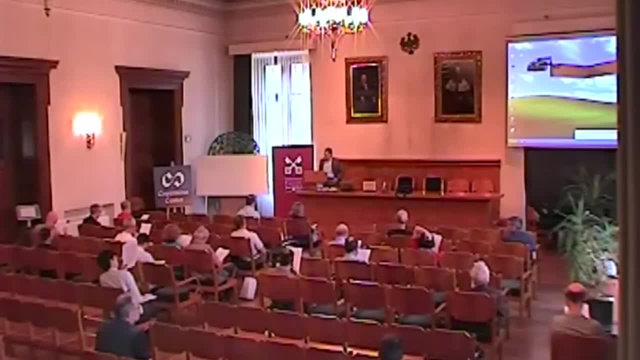 words that you understood perfectly well when I said them mean something other and secret that they supposed to understand. To capture those special intuitionistic meanings, the differences between their presumptive meanings and those of their conventional counterparts wholesale, we need, according to the anti-realists, 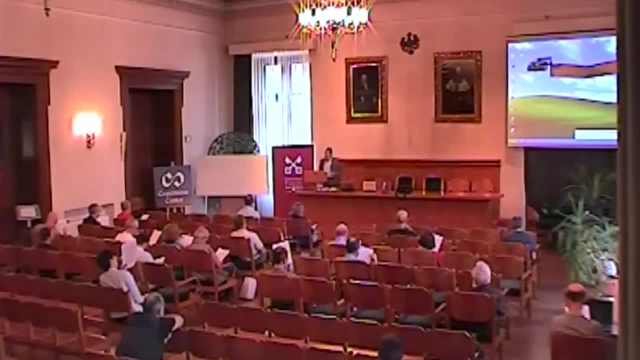 a new anti-realistic semantics. These anti-realists would have it that this semantics plays a role, with respect to intuitionistic logic and formalized mathematics, analogous to the role played in the classical case by Tarski's semantics and model theory, Page 6.. 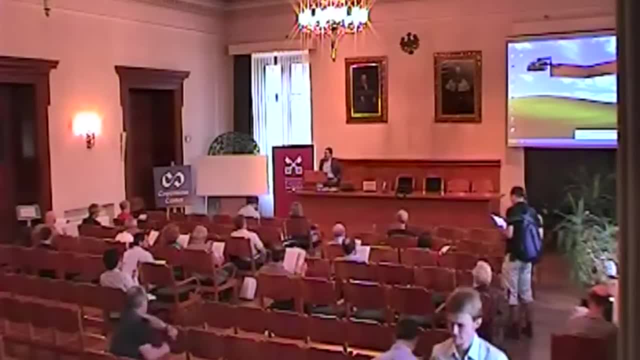 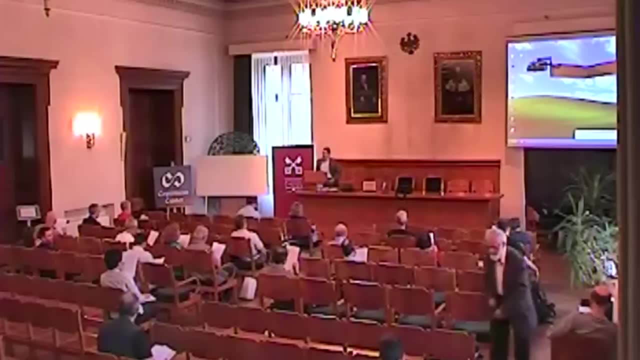 The trouble is patent. No one has ever provided a successful anti-realistic semantical theory for intuitionistic mathematics that plays the role of Tarski's model theory. There is a good reason to think that such a theory will never be forthcoming. A tiny fragment: 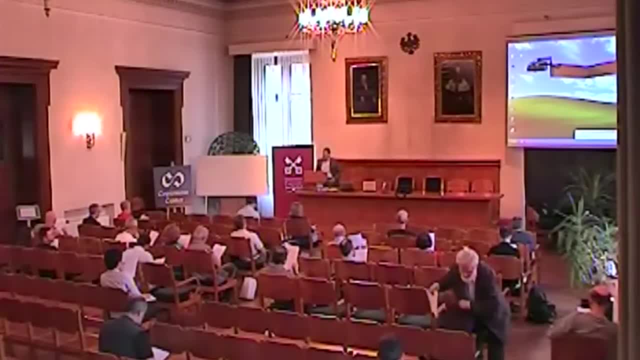 of intuitionistic set theory proves that intuitionistic propositional logic, not to mention predicate logic, higher order logic- is incomplete with respect to substitutional semantics. here you simply substitute names and expressions of theorems and Austria's E characters and names in for predicates- Tarski semantics of the usual kind, talking about structures and models. 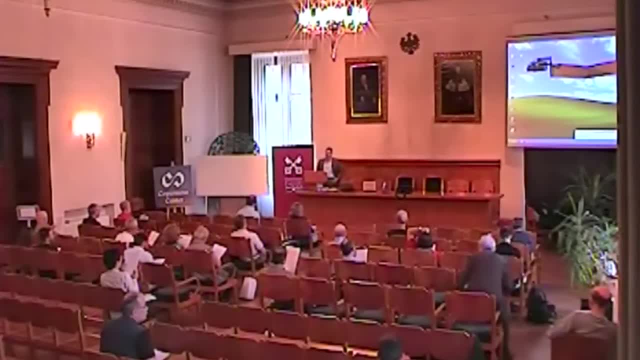 Kripke semantics and Beth semantics. So all of these are provably incomplete with respect to intuitionistic propositional logic. Finally, one more suggestion. Folks who should know better, among them Bill Tate, have turned their attentions away from the logical science. 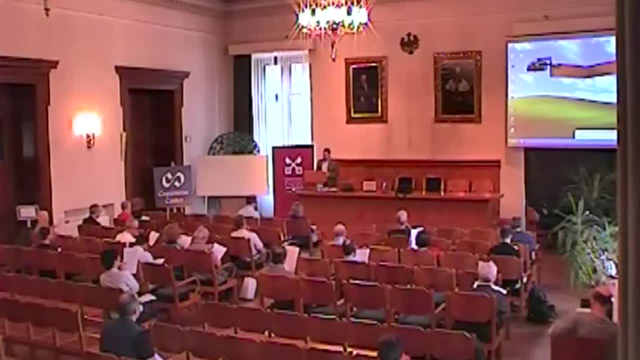 For them the culprit behind the differences between conventional and intuitionistic mathematics is mathematical, not logical. Some of them fasten upon the word function and its cognates. They would have it that the intuitionist means something else by the word function than is meant by conventional mathematicians. They demand that by the word 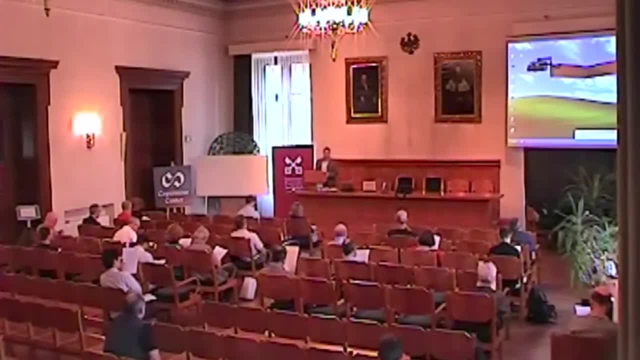 function. the intuitionist does not mean a collection of ordered pairs that are univalent in their second components. Once again, however, these functionalists are hard-pressed to say in any very definite terms what this new intuitionistic meaning is. Besides, I hasten to point out that if you consult any competent textbook on intuitionistic, 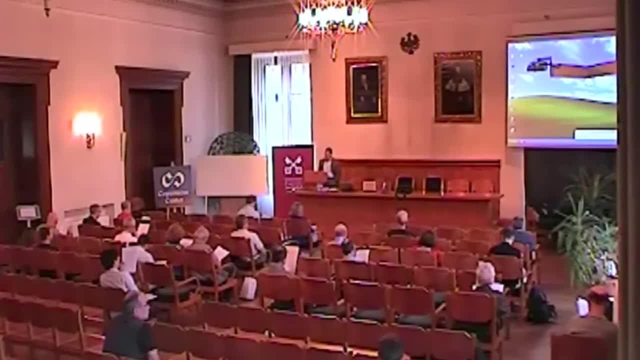 set theory, you will learn that by the word function, the intuitionist means nothing more nor less than a collection of ordered pairs that are univalent in their second components, just as you would learn from any competent textbook in conventional set theory. So much for my brief survey of recent silliness in the positivistic tradition about intuitionism. 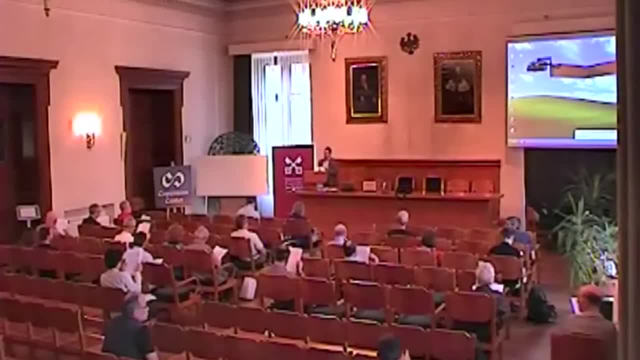 Now I've cleared the floor, Let's do something sensible. Page 7, something sensible: Today I console myself with deducing from the most basic idea of mathematical realism an outright contradiction. Now, this particular deduction is schematically An old and familiar, very old friend, if you like, a very old friend wearing a slightly new hat. 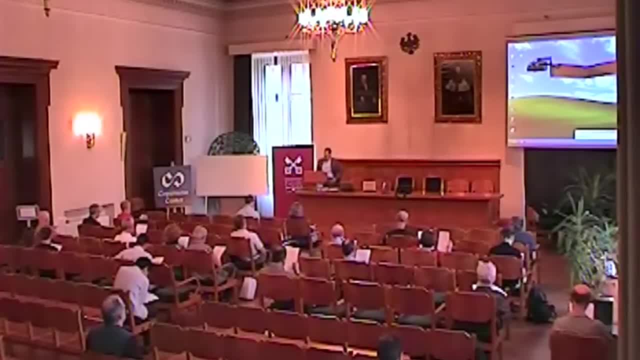 The deduction that it exists is not the point. Any high school kid could do this. One of my points is this: It's italicized, The deduction is in no way intuitionistic or conventional exclusively, but ought to be accepted by both those pugilists in the foundational slugfest. 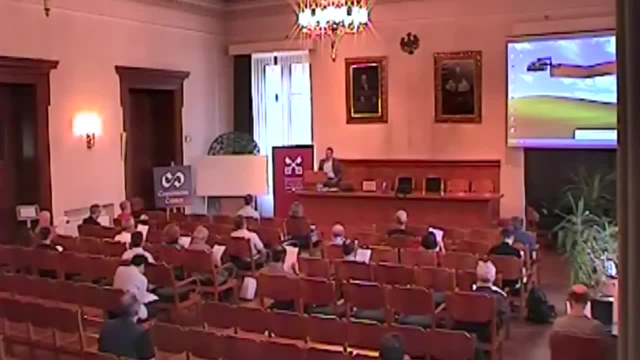 So everybody involved, conventionalist or intuitionist, needs to accept what I'm about to do. The second point is that the whole business offers a challenge to members of the audience who don't like the conclusion of the argument, namely that the thesis of mathematical realism 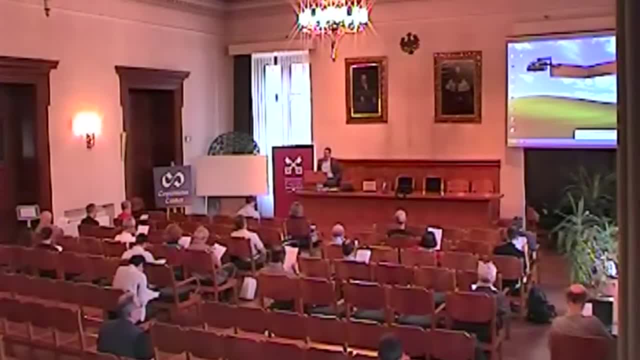 when added to some highly elementary mathematics, leads to an outright contradiction. Perhaps members of the audience who don't like that conclusion will help me out by explaining to me in detail and correctly where, at precisely what step, I've gone awry in the argument. 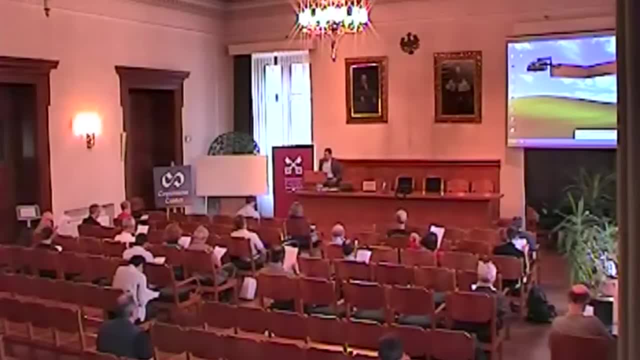 will explain to me exactly what fallacy I've committed and will tell me just where I have put one across. I have nothing up my sleeve except a debt to Richard Dedekind and his superlative monograph Was sind und was sollen gesahlen. 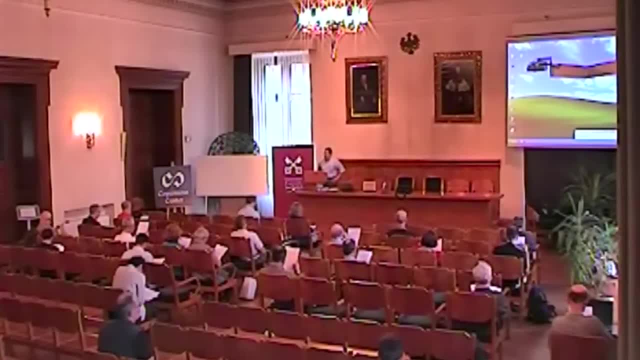 Here goes the deduction To start. I take this to be a central thesis of the mathematical realist. It's on the bottom of page seven. Generally put, mathematics, all of it- owes its great metaphysical and epistemic power over us to its truth. 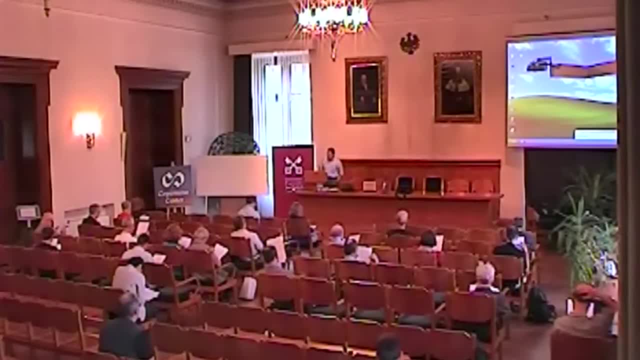 that is the truth of its theorems. That truth consists in mathematics' ability to report correctly upon the internal characters of various whatnots, as determined by the properties and relations, obtaining, among the page eight, components of those whatnots, components I call ding-dangs. 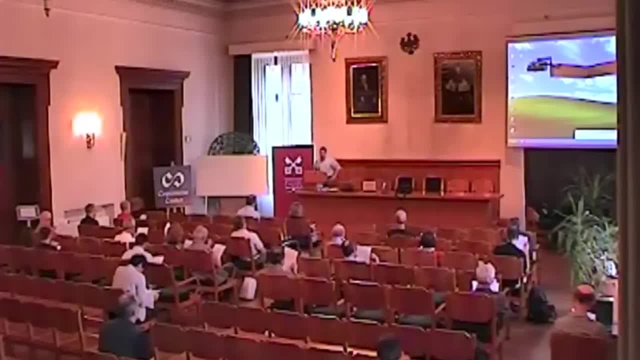 Now I'm not, or I am sorry, I'm not sorry, I am sorry if you've not been in touch with recent developments in the theory of whatnots and their component ding-dangs. The absolute need for such a neutral theory arises because mathematical realists, in their very stripes, 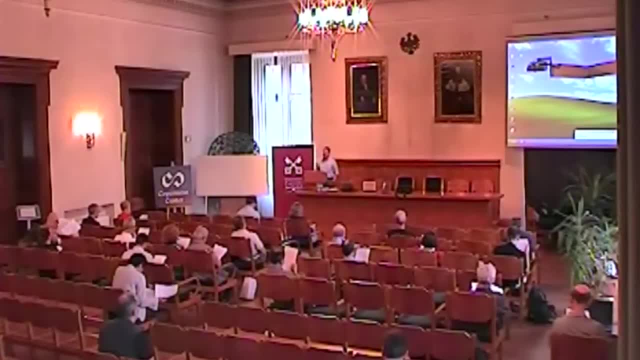 cannot agree one with another about the most elementary posits of their shared theory. Some would have it that mathematical claims are true in virtue of reporting correctly and exclusively upon the behaviors of sets and their component elements. Willard Van Orman Quine was one of these. 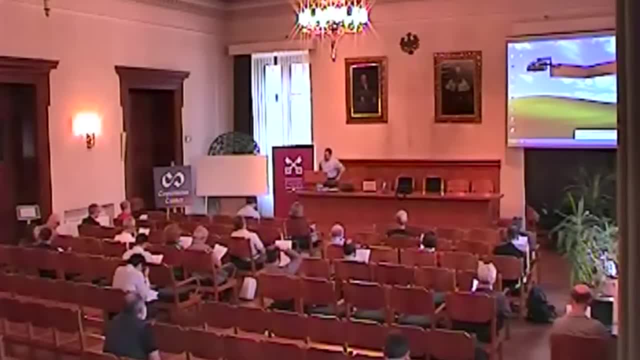 Other realists around here would have it that mathematical claims are true when they are by reporting correctly upon mathematical structures and the component positions in those structures. Yet others demand that no mathematical claims are true in virtue of reporting correctly on the goings-on in and among one or another of Eilenberg's and MacLean's categories. 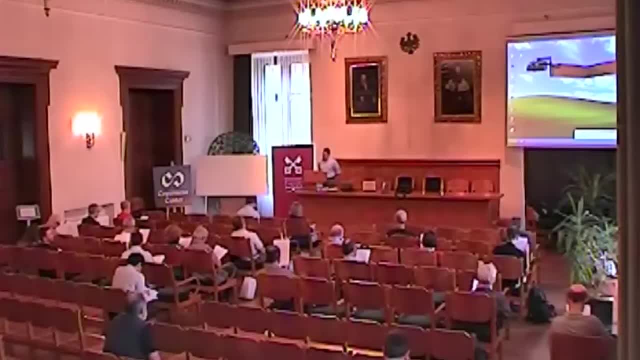 and the objects and sub-objects inhabiting those categories. There are even others that I won't list here. it's too boring. I shall therefore continue to refer, rather than to structures or sets or categories, to whatnots and their internal ding-dangs, rather than to sets and elements or structures and positions. 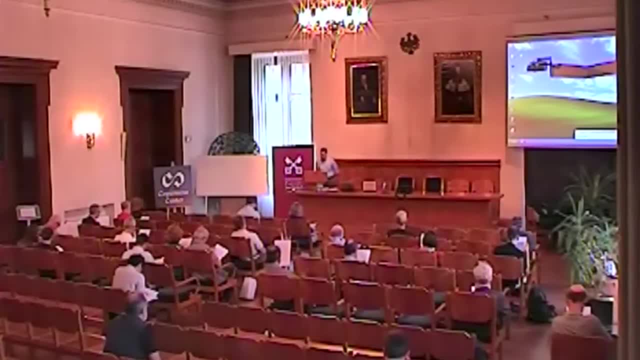 or categories and objects, because I do not even by implication wish to claim allegiance to any of these forms of temporary insanity, I have recourse, then, and only then, to a neutral theory of whatnots and ding-dangs. If you press me, I would have to admit that I am using the neutral theory of whatnots and ding-dangs. 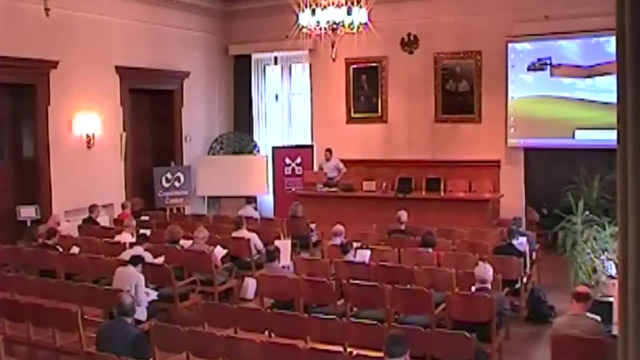 in this deduction, because I don't give a ding-dang what any of these realistically construed mathematical thingies really are or not. Now we go to work. What are the basic statements of a serious conventional theory of the arithmetic of the natural numbers? 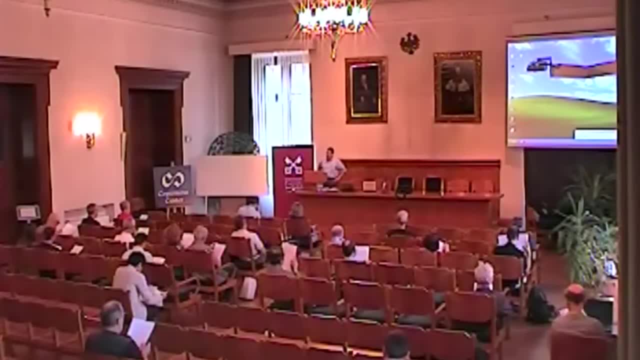 Page 9.. As primitive terms we have the symbol zero, the unary function s, the binary function symbols for plus times and capital E for exponentiation, which we all write infix, the binary logical relation symbol of two bars, also written infix. 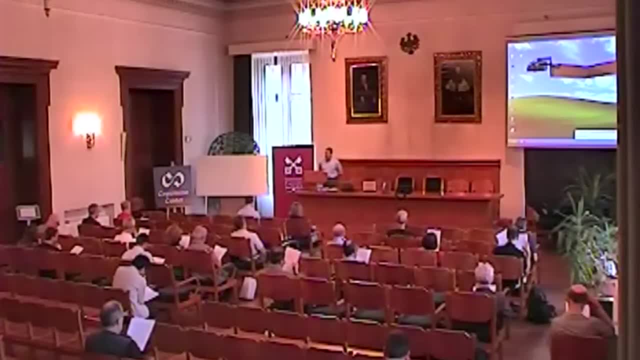 the individual variables lowercase, x, y and z, and the same again with natural number subscripts, x1,, y1, z1,, for example, and unary set variables capital, X, Y, Z, with numerical subscripts as well. From these, as is familiar, we form the usual compound terms, both close and open. 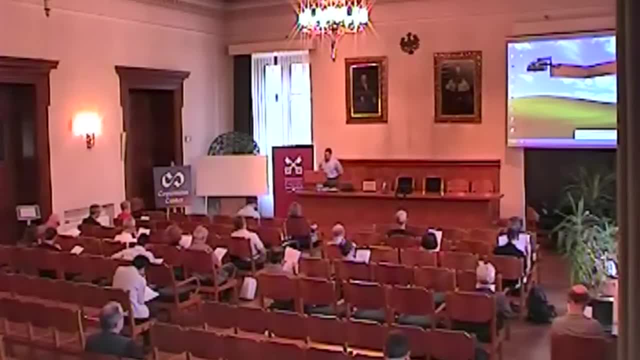 For example, S S S zero as a symbol is a standard syntactic. new number, S S S zero is a numeral for three. There are also computational terms such as S zero plus X, one plus X, if you like. 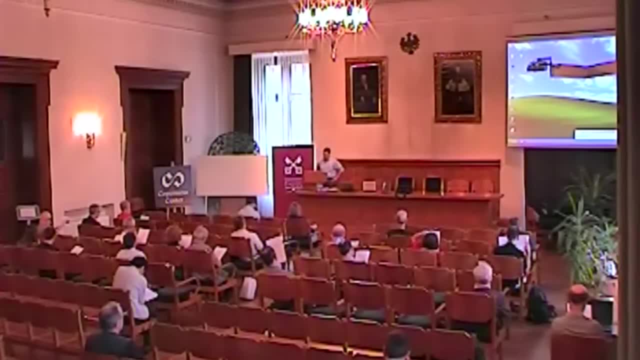 and X to the power, S zero, et cetera. From these in turn, using the double bar and set variables, we build atomic formulae, closed and open. The elementary sort of atomic formula is obtained by writing a term one, the double bar, term two: 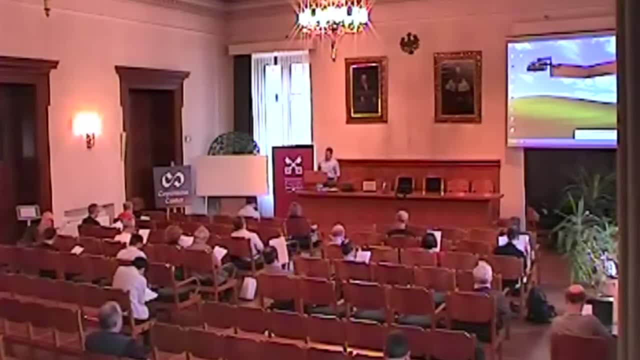 Just take two of the terms and put the double bar in between. For the higher order sort of atomic formula, we write a unary set variable followed by a term, For example X, followed by a term in parentheses. All this is familiar. Now we combine such atomic formula using the four standard connectives. 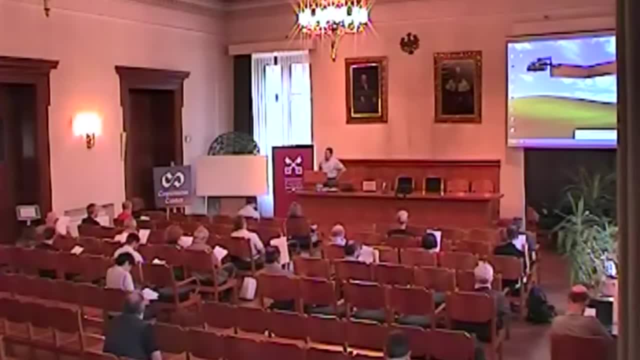 conjunction, disjunction, conditional negation and the two quantifiers, existential and universal, iterating each a finite number of times to obtain the class of arithmetic formulae, both open and closed. We allow unlimited quantification with both individual and set variables. 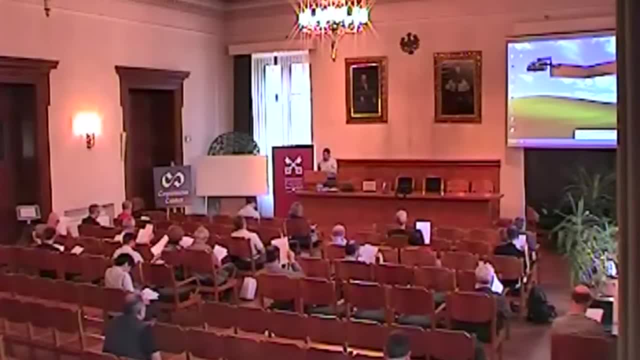 Again, all standard stuff. Among the closed formulae, we pick out those that qualify as axioms of the theory: Page 10.. Your glasses aren't broken. Page 10 came out in a different type font. Sorry about that. Those of you who had the bifocals, like me, will have to use the smaller. 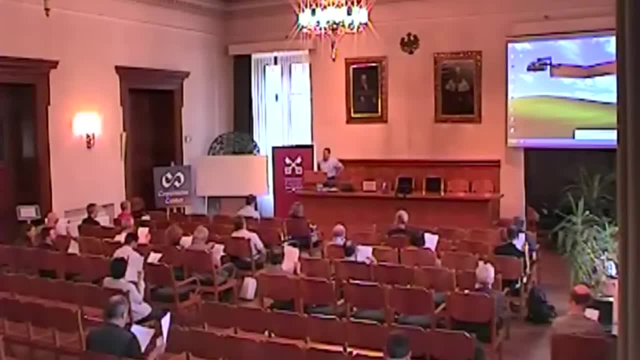 lower part of your glasses. First we have recursion axioms for successor terms. No number has a successor. that's zero. Numbers with the same successor are equal. Then we have the usual recursion axioms for addition, multiplication and exponentiation. 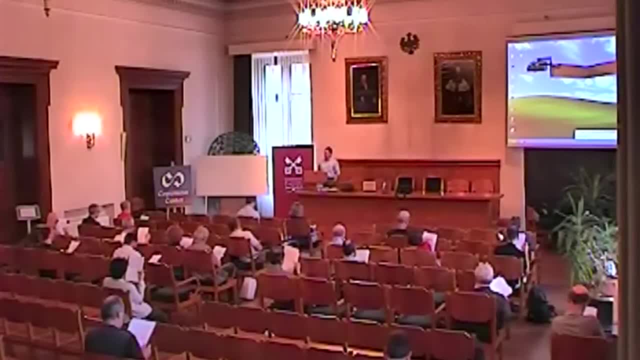 For example. for addition, add any number to zero, we get the same number back. Any number, X added to the successor of Y is the same as the successor of the sum of X and Y. Finally, we have full comprehension. That is, every definable property defines a set. 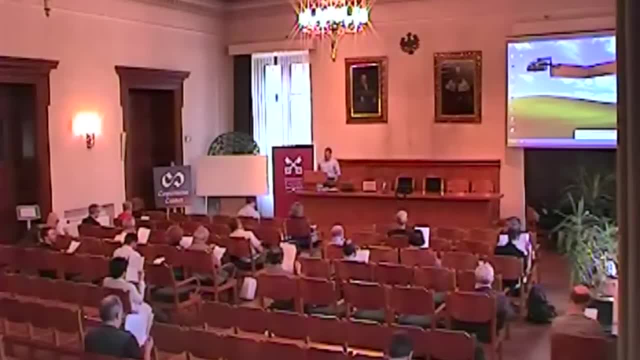 and a higher order induction on all sets. If a set X contains zero and is closed, under successor every number belongs to X. These are the axioms of, as everyone knows, second-order Piano, Datic and Arithmetic conceived of, for the moment, conventionally. 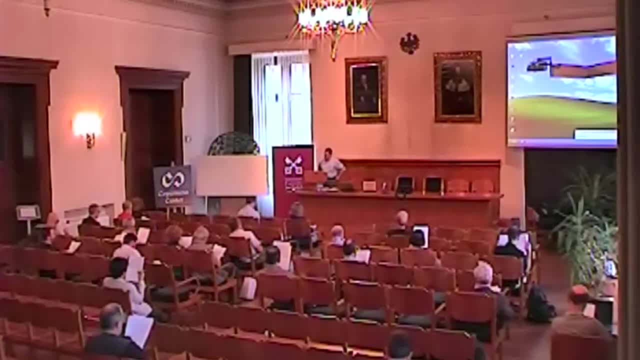 As everyone here also knows, it's a powerful theory in which one can formulate and prove all the familiar results of standard arithmetic and real analysis. One can show that the natural numbers are arranged in a well-founded linear order, with the zero thing as a least member. 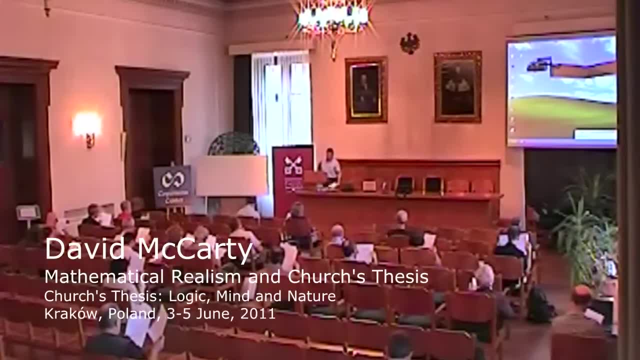 And one can formulate and prove- page 11, that the halting problem is unsolvable and hence that there are total functions- the characteristic function of the halting problem set being one of them- that are not Turing computable. In other words, Church's thesis. 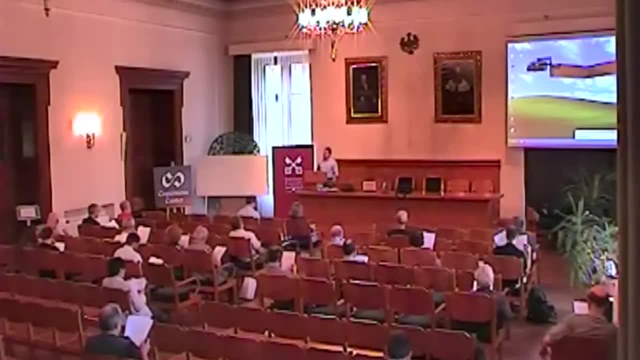 now I point out here that the statement of Church's thesis I'm about to give is intuitionistic Church's thesis. It has an extra half on it that the classical Church's thesis does not have. We'll come to that in a minute: The statement that every total function. 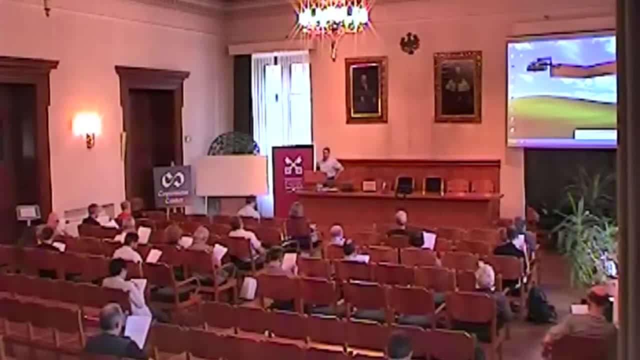 from the natural numbers to the natural numbers is Turing. computable is provably false on the conventional view of things, numerical. Next, I apply to this well-known and well-loved theory the basic principle of mathematical realism. So we know that there is a what-not. 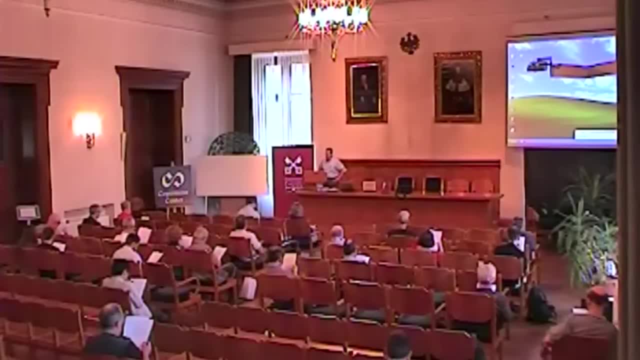 and that these axioms are true in virtue of reporting correctly on the situation in that what-not when it comes to its component ding-dings. For the remainder of the talk, we will call this the classical what-not and its components- classical ding-dings. 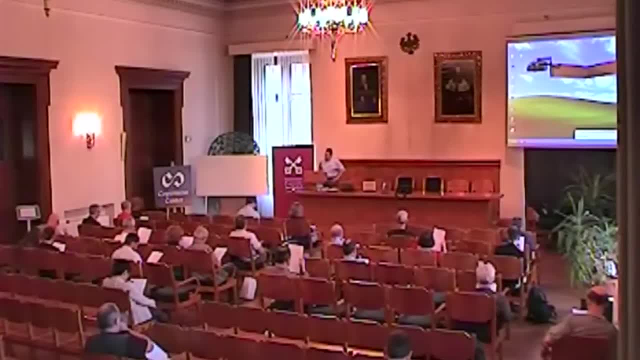 or a C what-not, and C dings for short, So that there can be reports in the arithmetical language. there are ding-dings in the what-nots denoted by the basic closed terms. There's a ding-ding in the C what-not. 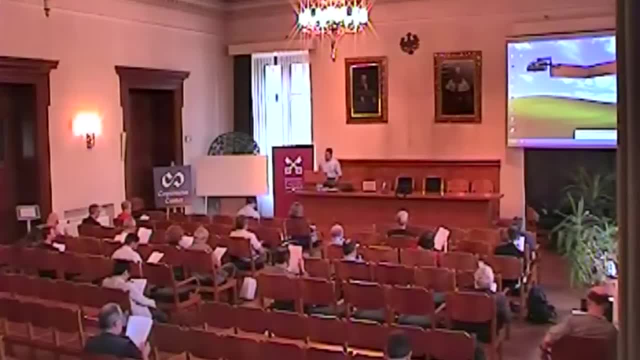 denoted by the zero symbol, and there's a unary operation on the C- what-not denoted by the S symbol- and there's a binary relation of equality on the C dings denoted by the binary double-bar symbol, All quite familiar. 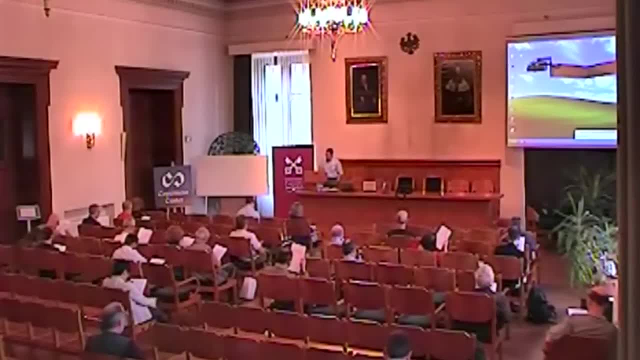 In the classical theory. we can prove that there are infinitely many C dings, that they are set into a linear order by the ding-ding operation denoted by S, that there is a least such C ding in the order it's denoted by the zero symbol, et cetera, et cetera. 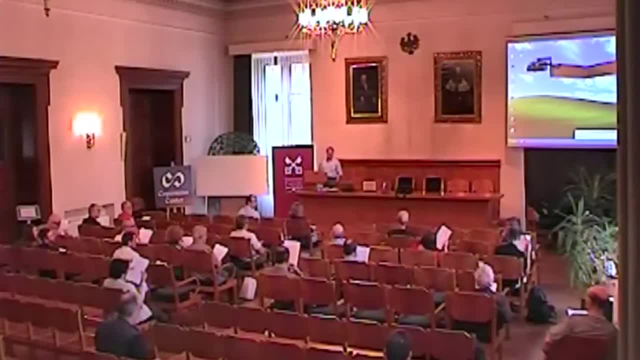 I'm sorry. Yes, Yeah, Thanks to the correct reporting of the induction axiom, we can reason up the induced order on the C what-nots using sets closed under the operation noted by S: All good, all well-known, all conventional. 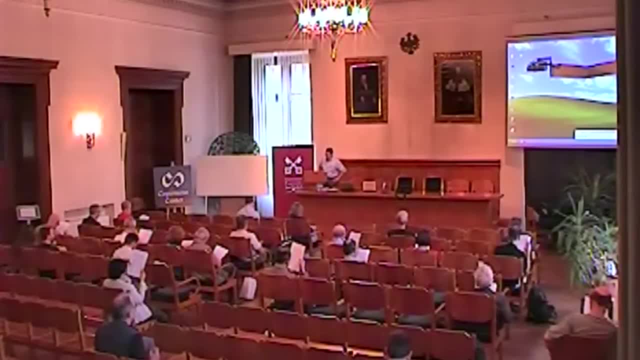 But now what about the shiningly brilliant intuitionist and his clever arithmetic? Up to a point it is very much the same story. The intuitionists have the same formal language of arithmetic- I must emphasize this- with the same primitive terms. page 12,. 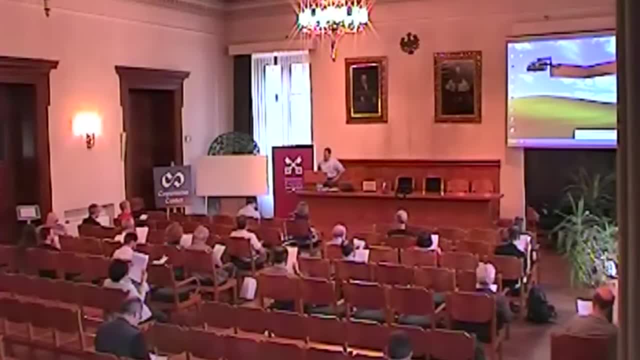 the same compound terms, the same atomic formulae, the same closed and open formulae. Further, intuitionists have very much the same axioms. Zero was the successor of no number. Numbers with the same successor are equal. The identical recursion equations governing the symbols. 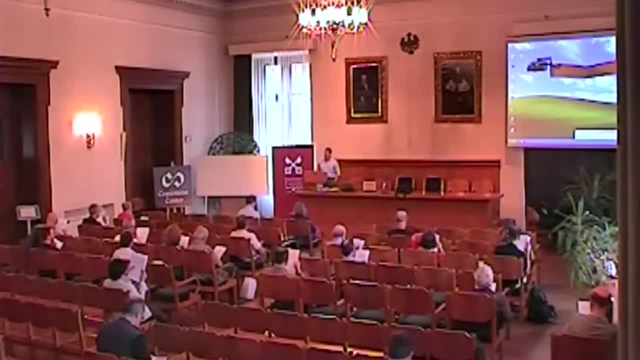 plus times an E, full comprehension and mathematical induction over all sets. Here we have at least one additional axiom. Church's thesis. the statement expressed in the formal language using formal renditions of Kleene's computation and upshot, predicates that every total function of natural numbers 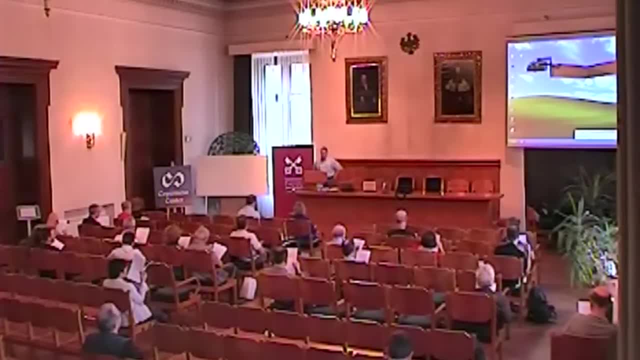 is Turing computable. There is also, by the way, something called the uniformity principle- I won't go into that today- governing all sets of natural numbers, but that will not concern us today, Since I'm addressing a conference on Church's thesis. 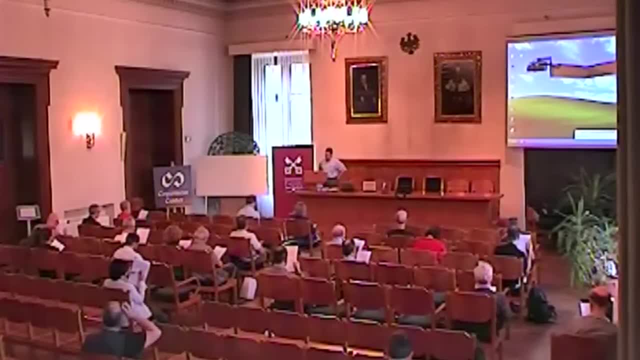 I ought to give some articulate reasons, if only in the form of sketches, to indicate why I think that Church's thesis is true and admits of proof. I have divided the reasoning into two parts, the first of which I take to be definitive. 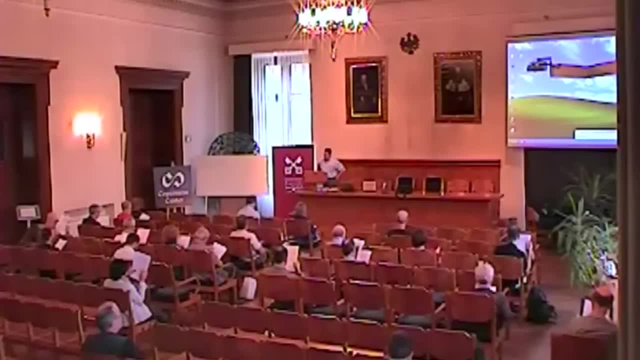 In that part I prove that every natural number function is humanly computable. For that I employ the mathematical assumptions. every proof starts with assumptions. here are some of mine, sometimes misdescribed as Heitink's explanations, which we can better describe as: 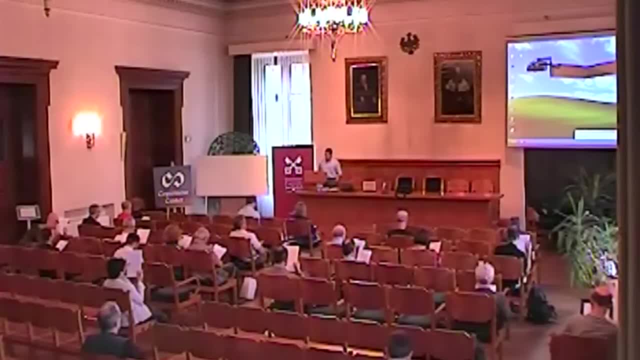 realizability with respect to humanly computable functions. The second part of the reasoning for Church's thesis, which is an argument for a statement first proposed by Turing, is predicated upon an assumption that I will describe when we come to it. Here is the first part. 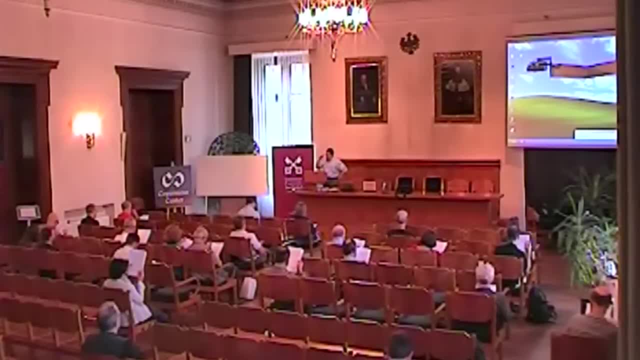 of the two-part argument. Let R be a binary total relation over the natural numbers. For every natural number x, there is a number y, such that Rxy. When such a statement is realized, we know that there is a humanly computable function f. 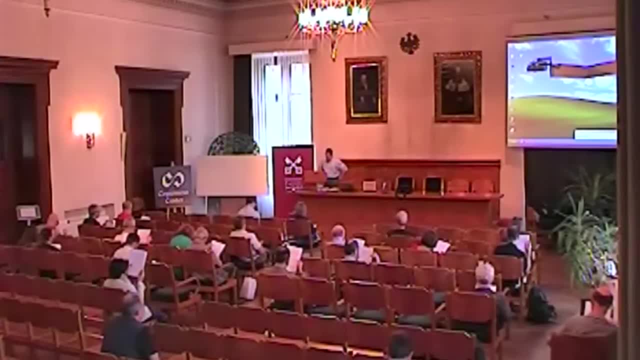 that is total on x and such that for every x, f on x realizes there is a y, such that Rxy- These are part of the assumptions- to say what it is for a construction or humanly computable function to realize a formula. 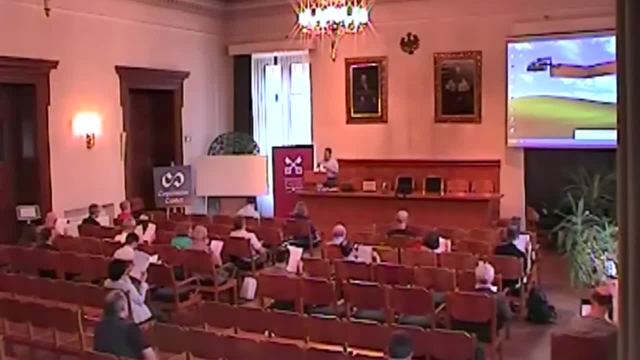 Realizability for first-order existential, page 13. quantification then allows us for every x to select such a y. That's what realizability tells us. Furthermore, there is a humanly computable function, g. therefore, that does the selecting. 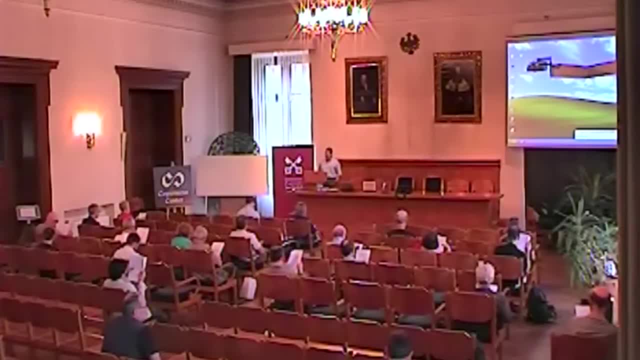 g is total on x, and such that for any x relation, R holds of x and gx in that order. And we are done. Every total binary relation of numbers is uniformized by a humanly computable function. We've laid down various axioms. 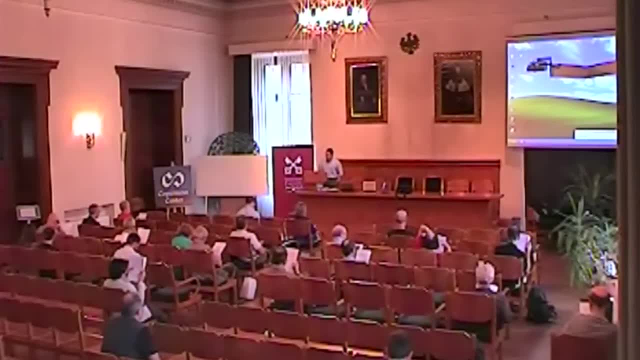 about what it is for a construction to realize a formula. Therefore, every total number theoretic function- each one of them is a total binary relation on numbers- is humanly computable. So ends the first and totally non-controversial part. 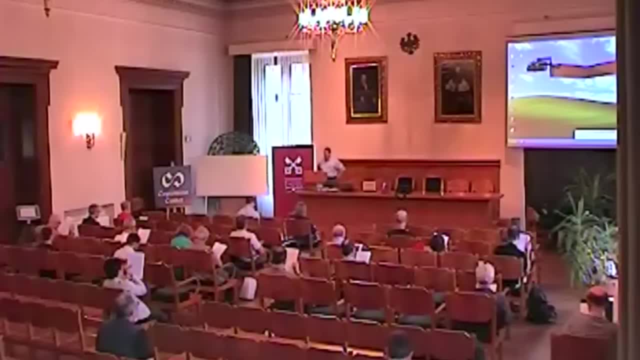 What about the second, more controversial leg of the argument, showing that every humanly computable function is Turing computable? For this there are a number of options, one of which might rely on Turing's analysis of human computation as set out in his justly famous 1936-1937 article. 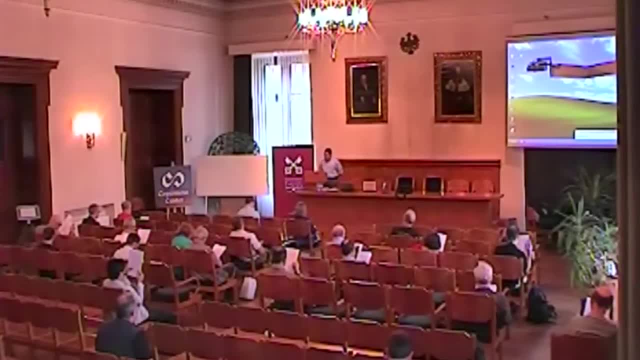 On Computable Numbers. As an intuitionist, I must be careful with Turing's argument and employ a constructive proof of the version of the Heine-Borel theorem, the theorem that Turing seems to have used to show that when inscribed in any closed and bounded square of paper, 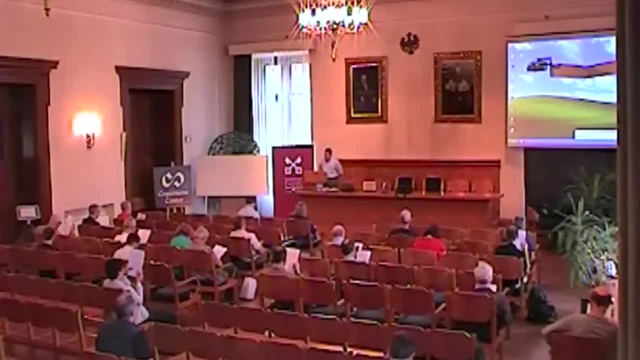 at most, a finite number of different symbols can be distinguished. There are intuitionistic proofs of the Heine-Borel theorem, some of which involve what are called formal spaces. Another option, more Gerdelian this time, would be to argue that there is a recursively innumerable 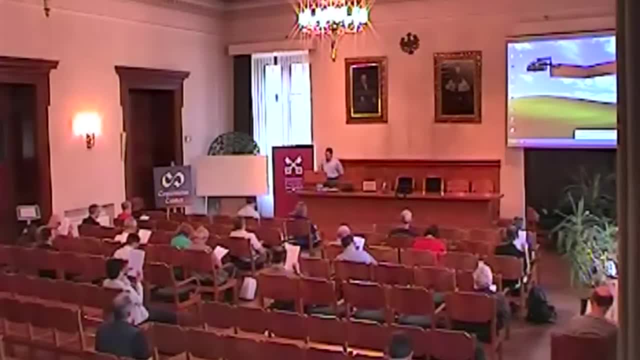 definitional extension, let's call it T- of ZF set theory sufficient under the needs of a theory whose algorithms humans can in principle tackle. Then, if F is a humanly computable function, there is an algorithm A, according to the instructions of which F is humanly computed. 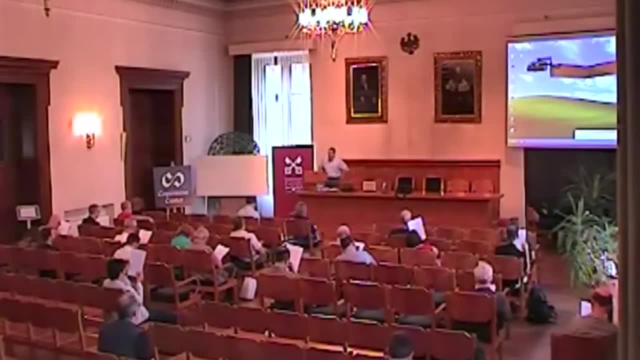 In the language of T. then there is a set theoretic definition, perhaps a denotational semantics, for the algorithm of A. call it capital D, such that for all natural numbers M and N, F outputs N on M, if and only if. 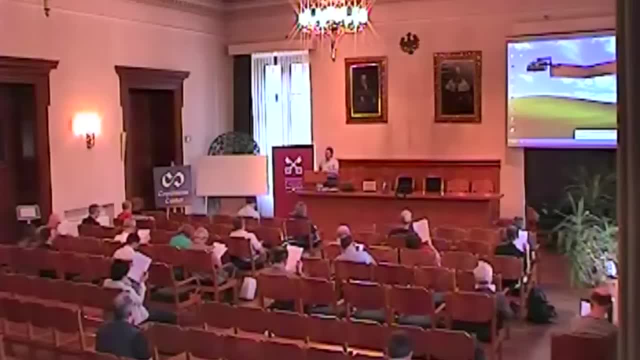 down at the bottom of 13,. algorithm A directs the human computer- thank you Wilford for that- to output N on input M if, and only if. page 14, there is a derivation T of DMN And the argument here is parallel to that. 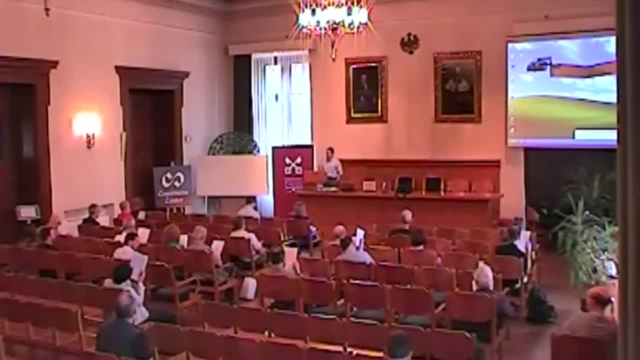 proving that every Turing computation can be defined in the language of elementary arithmetic and its action can be mimicked there by using derivation. Let me say parenthetically what this argument is. This: I take it to be part and parcel of the common claim that 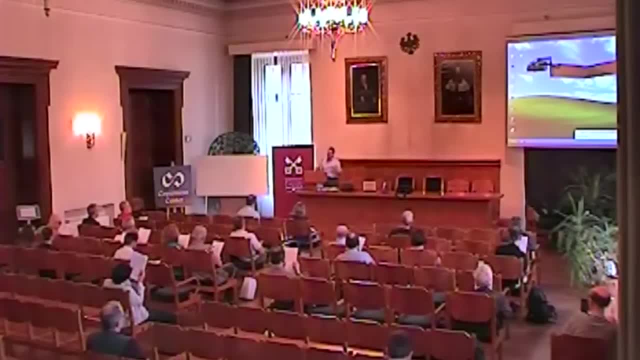 definitional extensions of set theory are sufficient under the needs of mathematics. If we take that seriously, that means that algorithms that can be carried out by human beings must be definable there, and we must be able, in detail, to prove their basic properties. 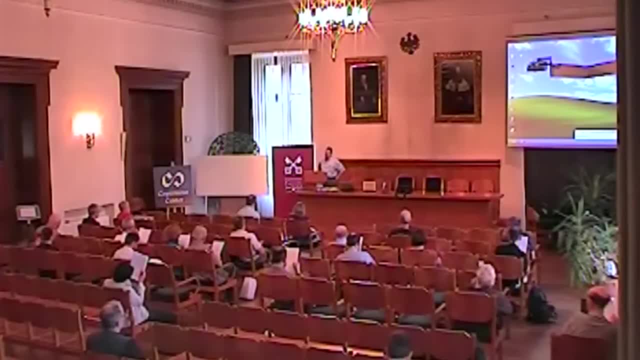 And so I'm arguing that they are numerically definable. and once they're numerically definable, we know that they're sigma-zero-one. Let's read on page 14.. As a result, the graph of F, the binary relation F of X, equals Y. 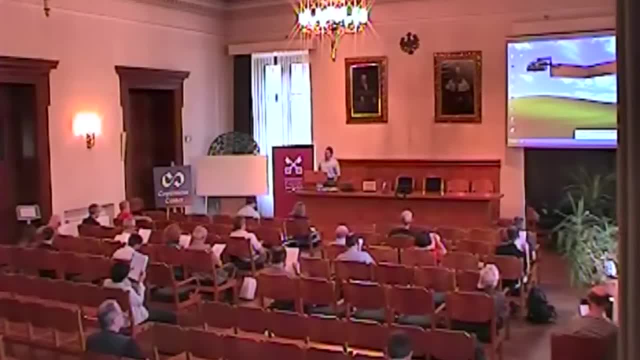 is extensionally identical to a sigma-zero-one predicate, The derivability predicate. it is derivable in T that DXY, X and Y are natural numbers. Notice: here T is not variable, here it is fixed. so I am arguing that there is a single definitional extension. 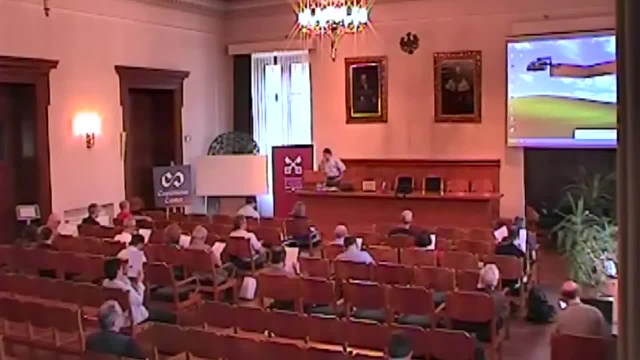 of set theory that's recursively enumerable, that has this property. Excuse me, Set theory is intangible since its graph is sigma-zero-one. Every humanly computable function is Turing computable, following this time from our claim that set theory had a certain completeness property. 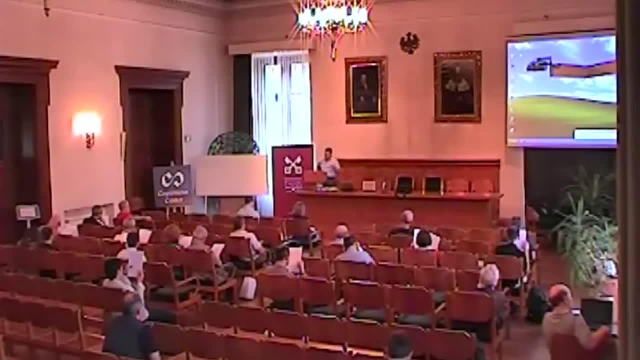 with reference to definition and proof, I should point out that this latter kind of encoding of a natural number algorithm into set theory, as well as the argument in Turing's paper, are plausible only on the assumption that one can faithfully encode a human computer into a finite number. 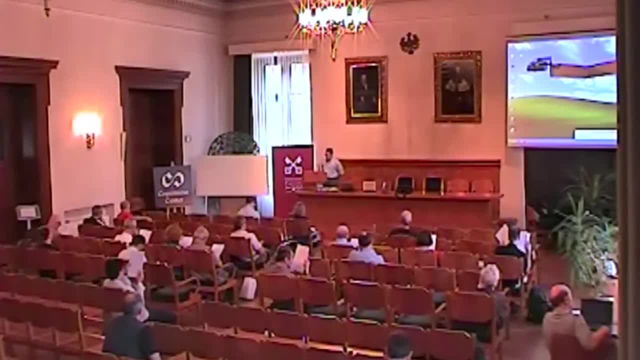 of finite states and hence into a single natural number. Such an assumption is subject to some controversy and at least to further investigation. I say parenthetically: To my mind, this may have been what Gödel was referring to later when he talked about human beings. 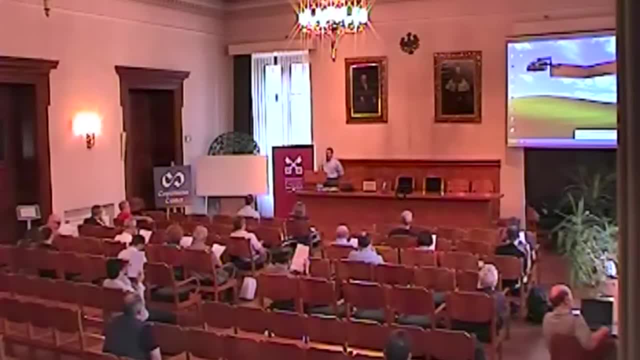 whose mathematical abilities will infinitely extend that of any Turing machine. Why is that? Because their relevant internal states do not constitute a finite set of internal states. By the way, I need not conclude from that that they constitute an infinite set of internal states. 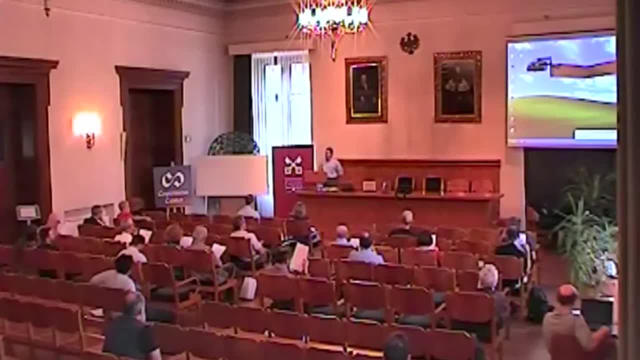 Do not commit the fallacy that every set is either finite or infinite. That is a fallacious claim even in conventional mathematics. Reading on, I can now return to the main Dedeck-Hindian argument. I will formulate that argument in terms of collections of ding-dings. 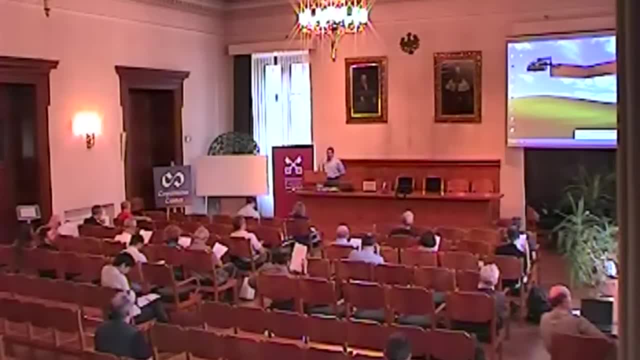 referring again to the classical ding-dings of the first order as C-dings, their intuitionistic fellows as I-dings First, I hope you will allow me a simplifying assumption that is inessential. No one will doubt that the I-dings 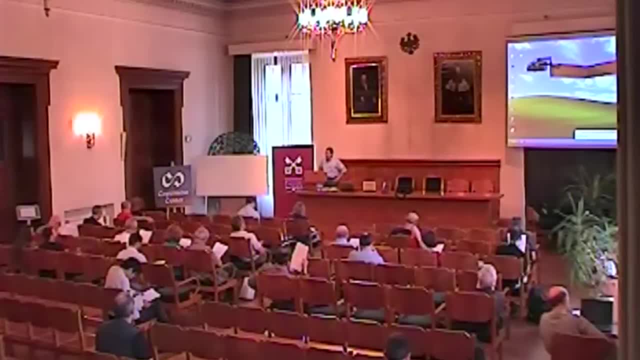 comprise a collection that is at most countably infinite and, in the usual time-honored fashion, can be faithfully embedded as a sub-collection of the C-dings. That way, we can work exclusively with the domain of C-dings, As can be proved in the classical theory. 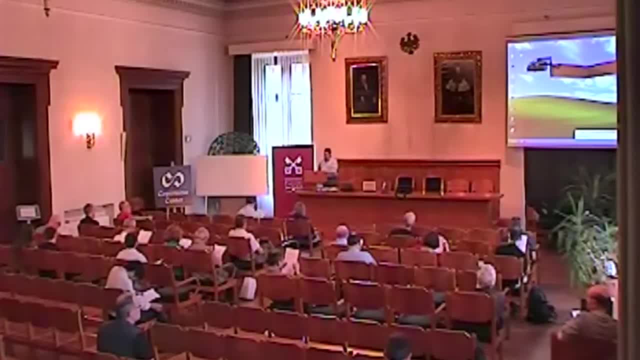 the C-dings are closed. under primitive recursive pairing, Pairs of C-dings can be treated as yet more C-dings. Let X be a collection of C-dings and say that a collection X is good provided that it contains the pair zero-classical-thing. 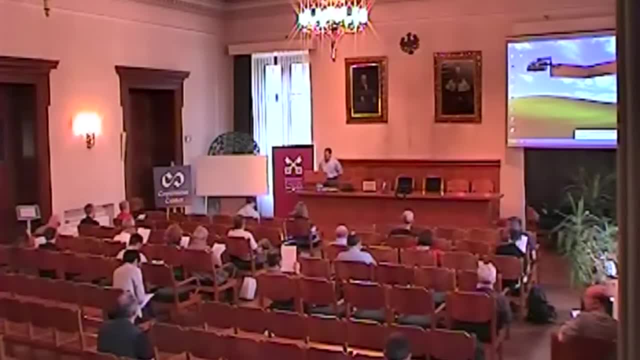 zero-intuitionistic-thing. it has a largest pair in it. its pairs are functional: that is single-valued in the second component, injective, that is single-valued in the first component, and back-inductive. What do I mean by back-inductive? 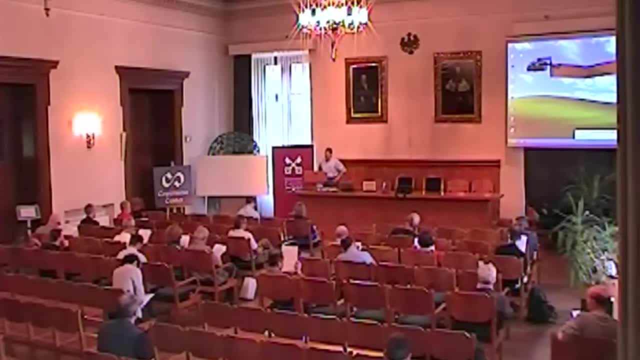 By back-inductive I mean that whenever a pair in X consists of a classical successor of A and the intuitionistic successor of B, then X also contains the pair AB, So it can strip off one successor from each one. It is child's play to show by induction. 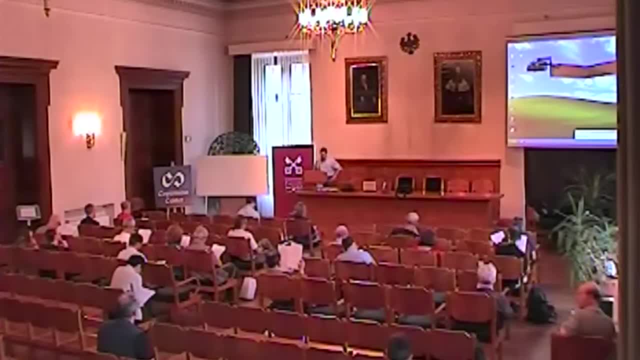 the union of any good collections is also good. Just as I do not have to work with the category of pairs of things, I don't have to work explicitly with finite collections or functions either. In both classical and intuitionistic domains, I can use powers of two. 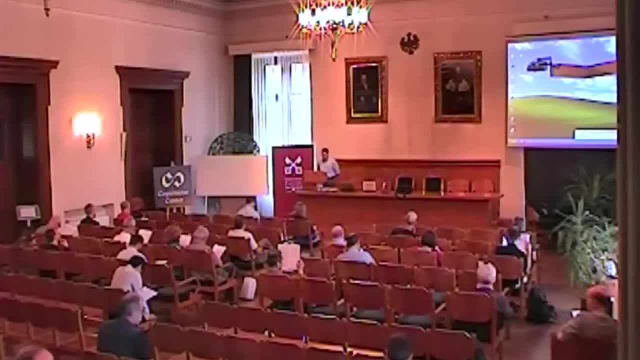 or binary notation to encode finite collections On this account. for example, as we all know, a finite collection, the triple set, unordered, 2, 3, 4, is represented by 2 to the third power plus 2 to the fourth power. 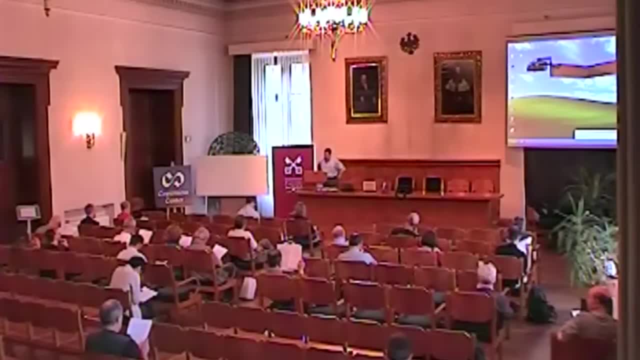 plus 2 to the fifth power, I can now use the existential quantifier in the classical theory to define what will prove to be a single function between the classical dings and their intuitions to counterparts in their respective domains- whatnots? 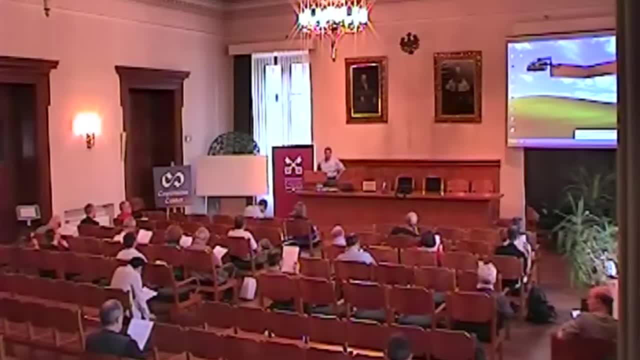 I'll call the function capital F and say that a C thing is related to an I thing C thing, A is related to an I thing B if, and only if, there exists- there's my existential quantifier- a C ding encoding a good collection and the code of the pair A- B. 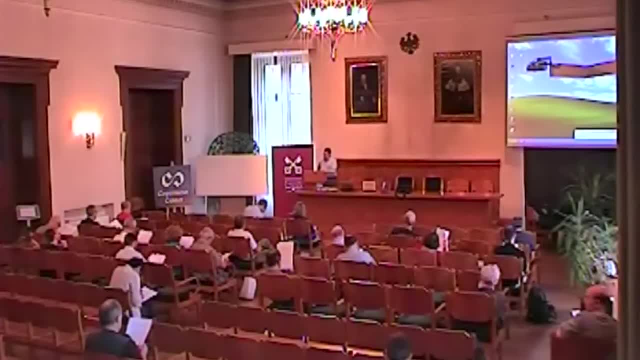 is in that collection so encoded. That is my very simple definition of the relation capital F, Page 16.. It's also a very simple matter to prove that F relates the C thing 0 to the. I ding 0, takes 0 to 0. 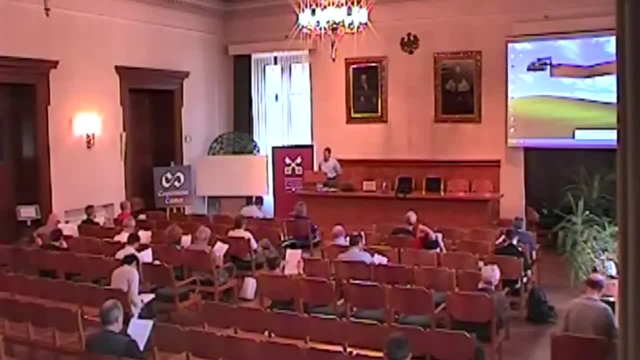 F is functional and F is injective. For those latter two, one uses the proven fact that unions of good collections are good To show that capital F is a total function. on the C things, one uses the classical principle of induction reigning supreme over. 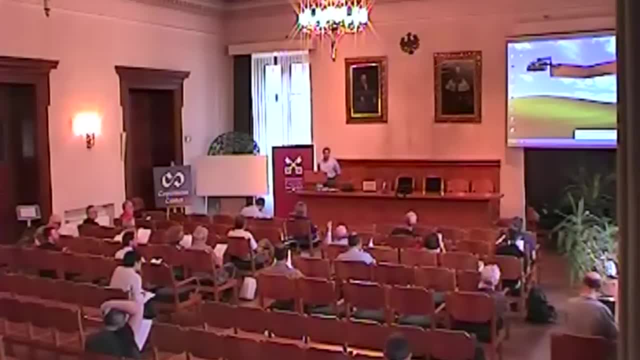 the classical whatnot throughout To show that capital F is in. I'm sorry, You talk about arbitrary union? Yes, sure. So how can you put something in induction if you talk about arbitrary units? I've reduced the arbitrary unit to an existential quantifier. 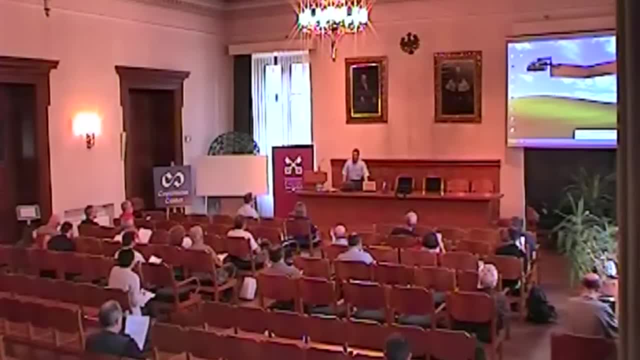 Now I'm encoding all the finite sets and then I'm simply quantifying over them existentially. Second, since I have second order induction, it doesn't matter whether I can define. I've actually done it. it doesn't really matter whether I can. 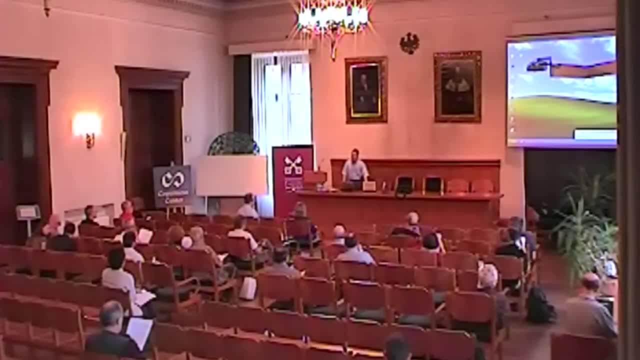 define the induction predicate. in the theory It is a set. So my second order induction doesn't require that I define it. I'm quantifying over all sets To show that the capital F is a total function on the C things one uses the classical. 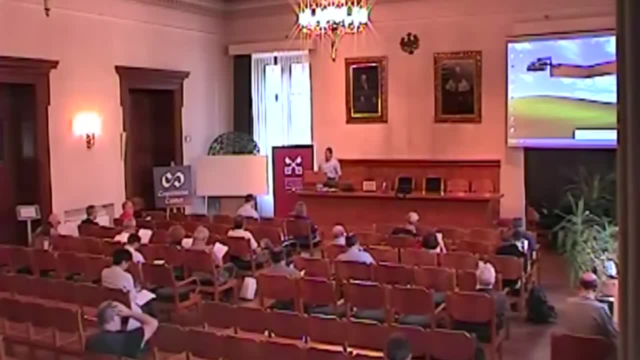 principle of induction reigning supreme over the classical numbered whatnot? domain. To show that capital F is surjective on the I things, one uses the intuitionistic induction. Therefore, the relation given by capital F is proven to be a total bijection between the first. 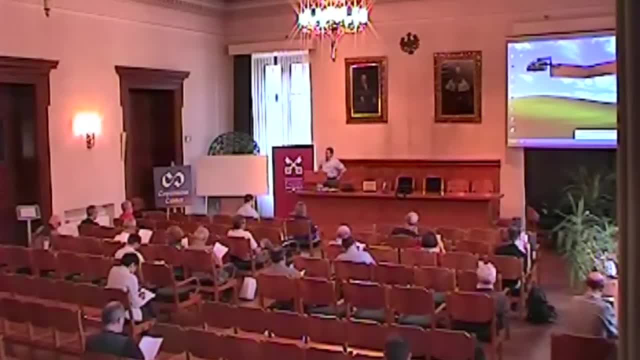 order part of the classical whatnot and that of the intuitionistic whatnot. None of this proof is objectionable either to intuitionists or to conventional mathematicians. Next, it is easy to show that the function capital F is also an isomorphism. 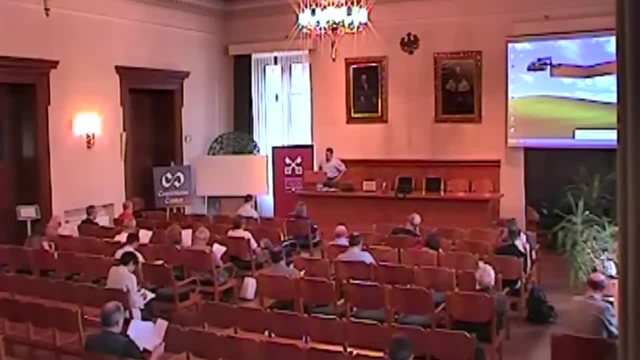 from the classical to the intuitionistic whatnot or domain. We've already seen that F takes the classical zero into the intuitionistic zero and that it commutes with the relevant successor functions on both the classical and intuitionistic sides to complete the proof of the isomorphism, as is familiar. 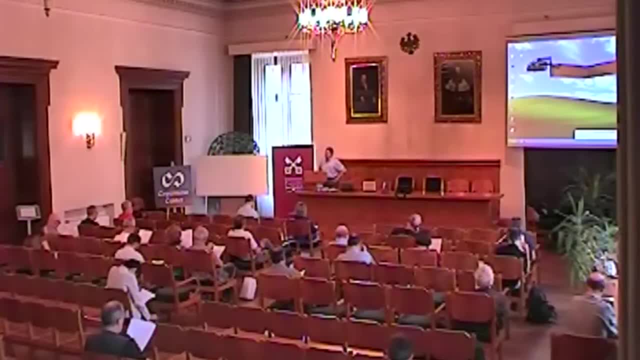 when one uses the recursion axioms for plus times and exponentiation. Finally, a proof by induction on formulae: both theories partake of the same class of formulae after all- shows that truths are preserved and back-preserved via the isomorphism capital F. 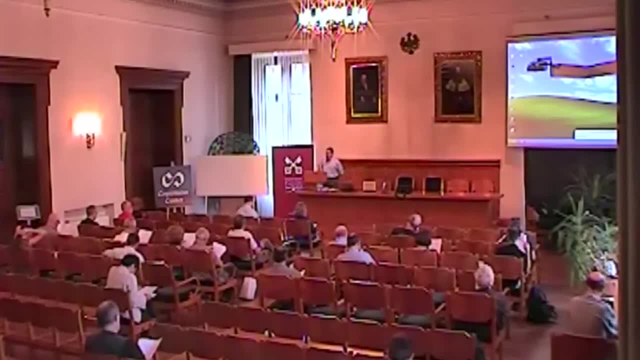 between the two whatnots. So if a formula phi holds of a classical thing, A in the classical whatnot, then phi holds of F of A, which is the intuitionistic thing in the intuitionistic whatnot, and conversely. Hence every truth. 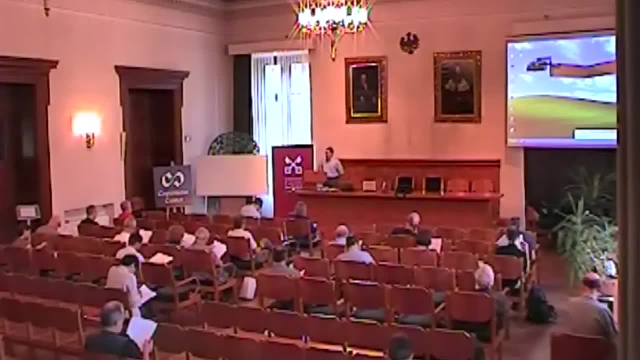 about the intuitionistic natural numbers holds of the classical natural numbers and conversely. By the way, this induction proof isn't really necessary, because all I'm going to do is show that the single formula that holds in the intuitionistic case also must hold in the classical. 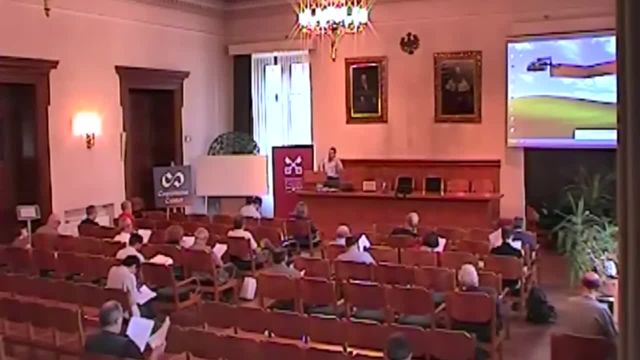 case. So I don't need full induction on formulae. All I would have to check is that the isomorphism respects truth up through a finite number of connectives and quantifiers. Therefore we have a contradiction. Church's thesis, the intuitionistic one, if we have seen. 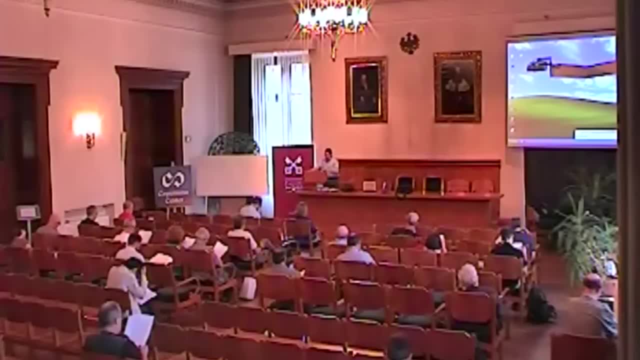 holds in the intuitionistic domain or whatnot, and so, by isomorphism, it holds in the classical or conventional whatnots. Hence it is true of the conventional, page 17 whatnots, that every function is Turing computable, But at the same time the 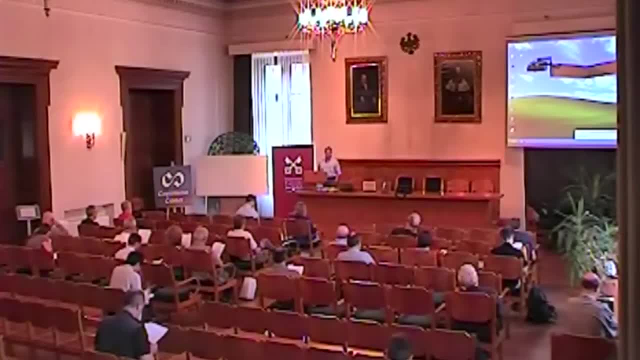 conventional mathematician, like my colleague Professor Abramson, thinks to prove that Church's thesis is false and that some functions on the natural numbers, such as the characteristic function of the halting problem, are not Turing computable. So ends the main business of the day QED. 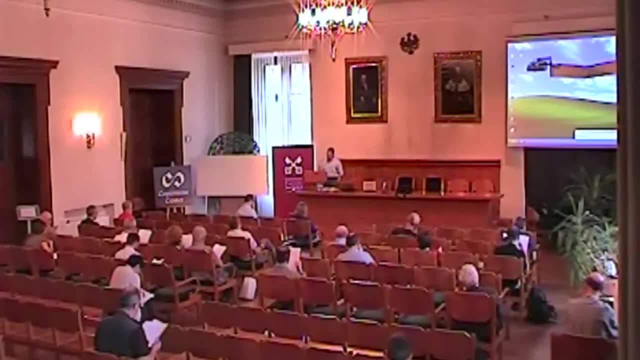 But now, before I yield the floor to questions and objections, I would like to say a few words that may cut some potential objections to my form of argument off at the pass. First, it's a mistaken objection identity. Someone might object that I have assumed that the same identity. 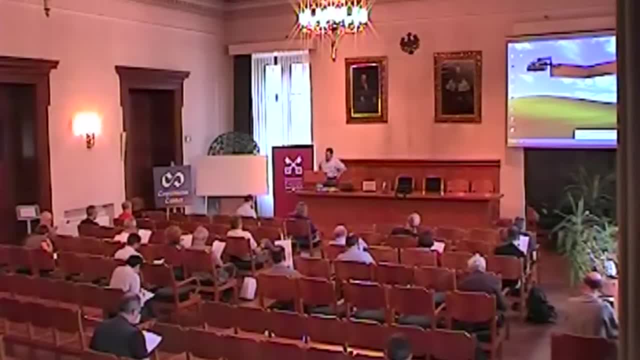 governs both the conventional domain or whatnot, and its ding-dings and its intuitionistic cousin. when I am not entitled to that assumption, I respond that such an assumption is inessential. Each of the two theories, just the formal theories, conventional and. 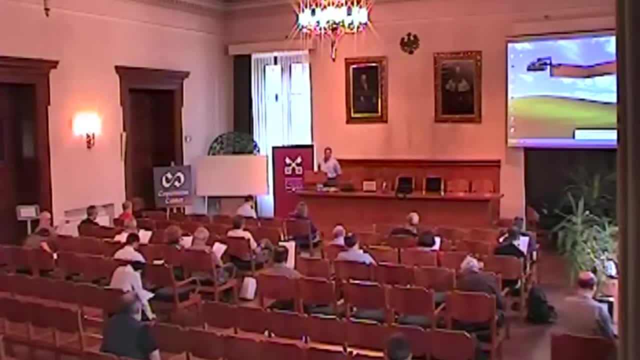 intuitionistic contains a suitable sub-theory of identity as part of the underlying logic And on the basis of those I can assume that the double-bar relational sign in the conventional theory denotes an equivalence relation on that whatnot, and the same thing for the intuitionistic. 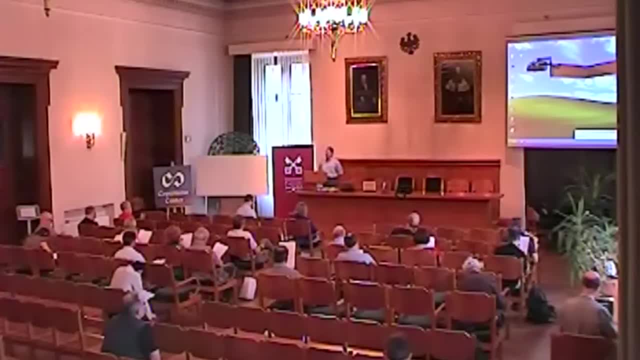 theory and its correlative whatnots. Both theories prove the theorem that the double-bar relation, whatever it is, must be reflexive, symmetric and transitive. Then I just take equivalence classes for the two relations. Very simple, This gives me a single identity relation. 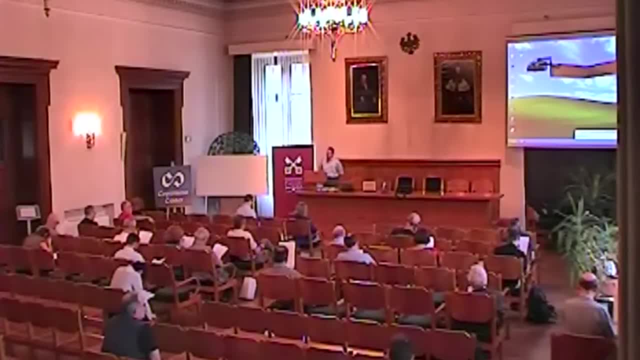 covering each whatnot, and I proceed as before. Second mistaken objection: Someone might argue that to prove that isomorphisms preserve and co-preserve truths, I must assume that the intuitionistic quantifiers commute with the relevant reporting upon predicate, That is, 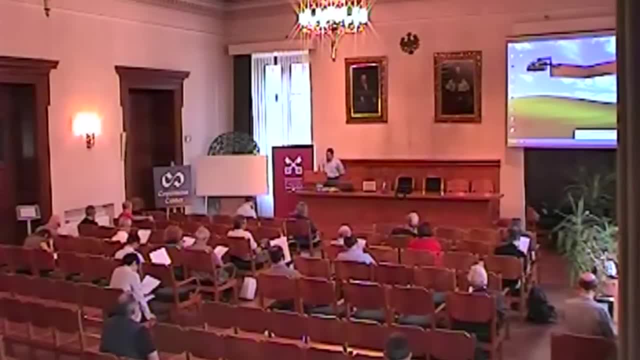 I must assume that the intuitionistic domain or whatnot satisfies the arithmetic formula. There is an x such that A where A is an open formula. if, and only if, there is an intuitionistic ding B, such that the intuitionistic whatnot satisfies. 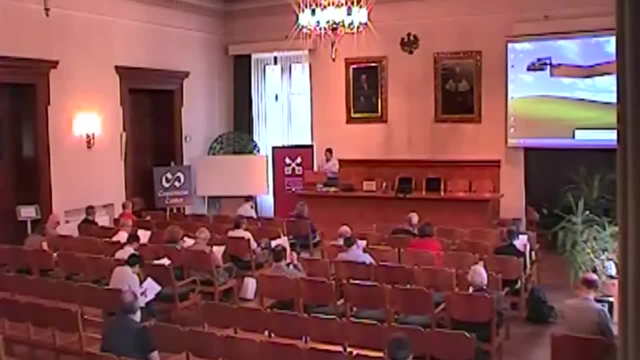 open formula A with x naming B And that this familiar Tarskian principle- page 18, is not correct for intuitionistic existential quantification. This objection also fails The claim just cited, namely that the whatnot or domain satisfies there is an x. 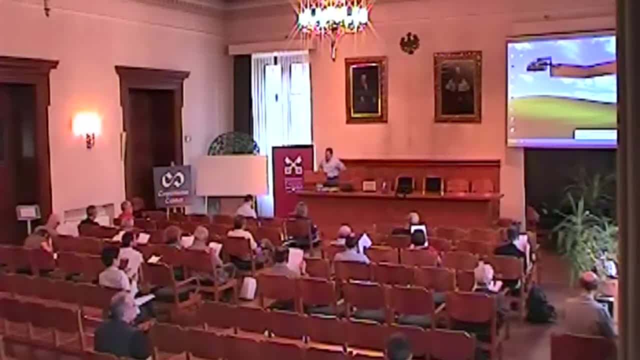 such at: A, if, and only if, there is an intuitionistic thing. B- such that the intuitionistic whatnot satisfies A with x. naming B represents standard intuitionistic practice and is used repeatedly, among other things, to justify intuitionistically the rules of intuitionistic existential quantification. 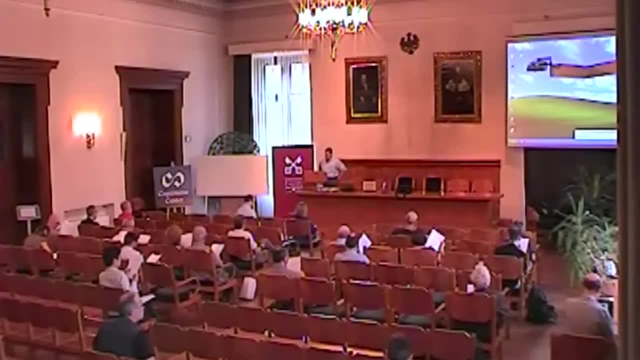 And, as we have said, these are the very same rules as the conventional rules. I should also remark that these Tarskian clauses for existential universal quantifier are provable from Heiting's explanations, or what I called the realizability definition for human computability. 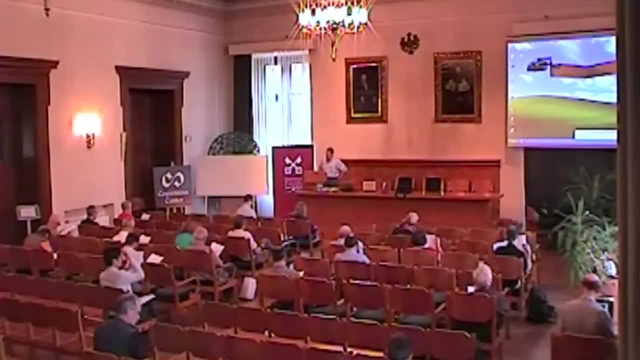 Some final remarks. Number one, One of the philosophical conclusions I'm not claiming it follows validly, but to which the argument of the present lecture leads me, I think, is this: There are no ultimate interpretations that stand behind all conventional and intuitionistic mathematics. 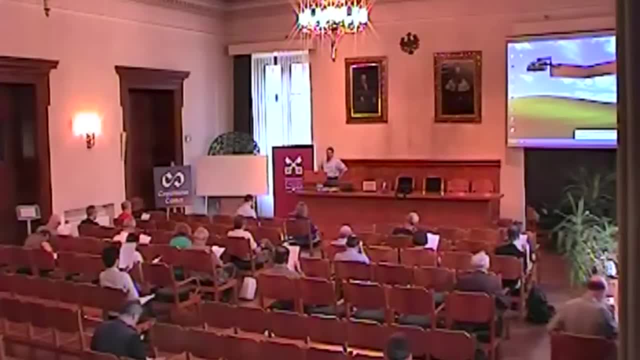 Philosophers and other well-intentioned folks are wholly unable to tell us finally and univocally what the terms in the mathematics mean. They cannot tell us whether they refer, in the last analysis, to sets or to categories. Further, there is no ultimate meta-language. 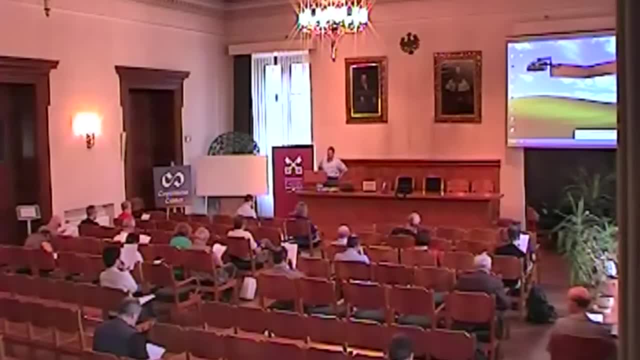 neutral between conventional and intuitionistic mathematics. This is something that Carnack very much wanted- In which those interpretations can be presented. You can't breathe in a space, outer space, where there is no air. Number two, In many ways, the lecture you have. 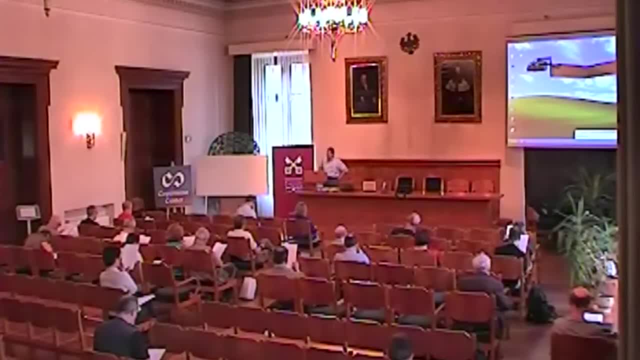 just heard is a tribute. It's a tribute to a prescient mathematician of the 19th century. His name was Paul du Blas-Rameau. Du Blas-Rameau was the brother of a famous physiologist, Paul du Blas-Rameau. 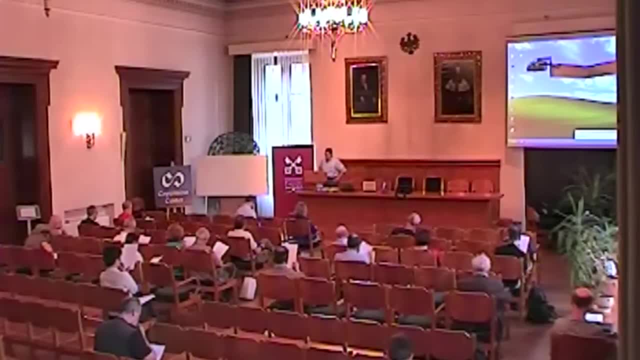 Like his brother Paul du Blas-Rameau, maintained that mathematical science exhibited what they both called ignorabimus. Hilbert liked to rail against ignorabimus In his monium opus Die Allgemeine Funktionen Theorie- General Function Theory- of 1882,. 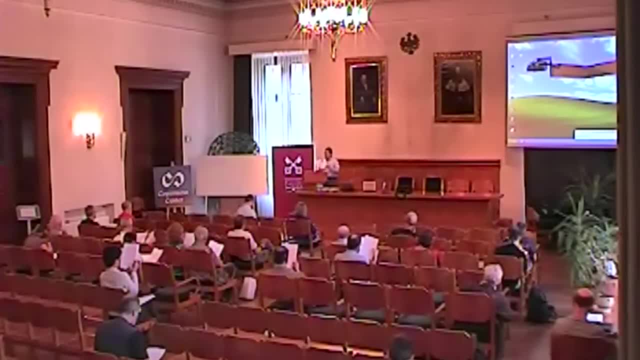 Paul du Blas-Rameau maintained, among other things, that mathematics- page 19,- manifests ignorabimus within its boundaries, That there are explicit contradictions and no foundational work of the future will ever be able to eliminate them in any way. Of course du Blas-Rameau did not have 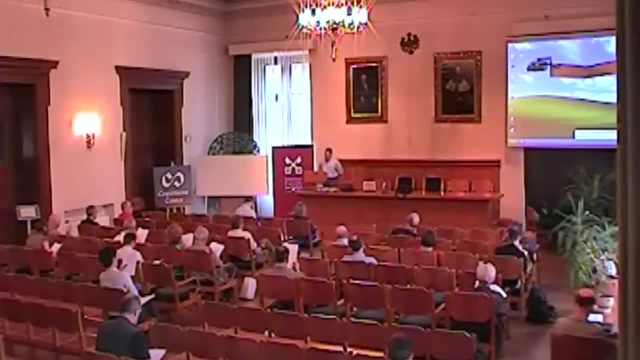 Church's thesis, or what I call the uniformity principle, in mind when he thought and wrote of ignorabimus, For example, he thought that the question- are there infinitesimals among the present standard reals of the continuum- represents a problem that would be unsolvable. 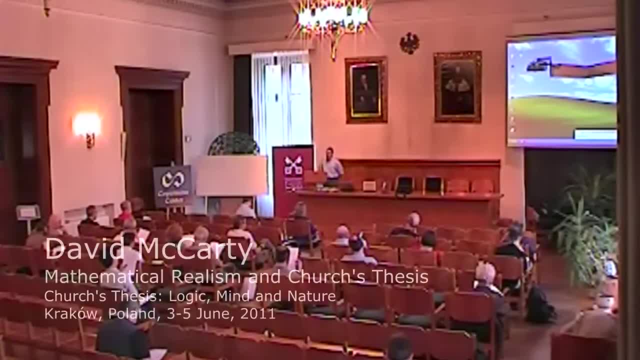 Some mathematicians contradicting others on that particular topic, Some arguing that there are infinitesimals, others that there are none. Now we know, on close analysis and from hindsight, that du Blas-Rameau got a number of things wrong and a number of things confused. 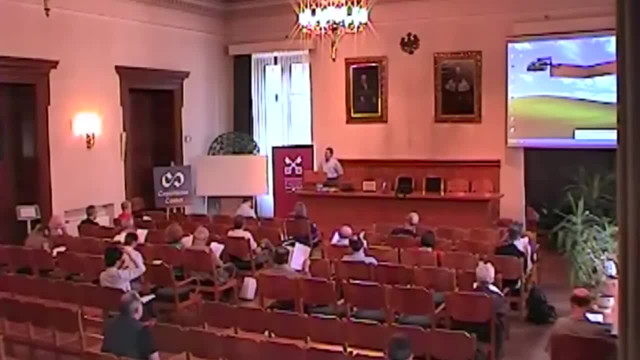 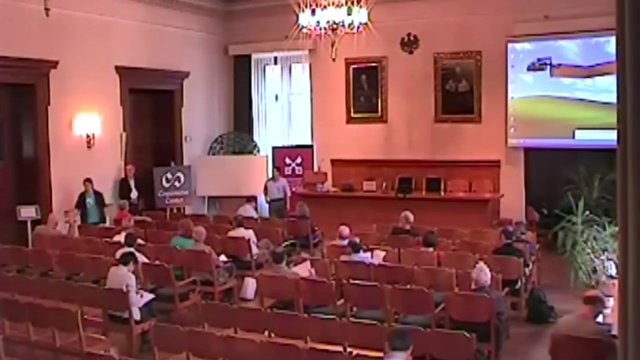 But I believe he did not get this part wrong, Hilbert. to the contrary. I'm sorry, Wilfred. in mathematics there is ignorabimus and plenty of it. Thank you very much for your kind attention. I have a question concerning this assumption. 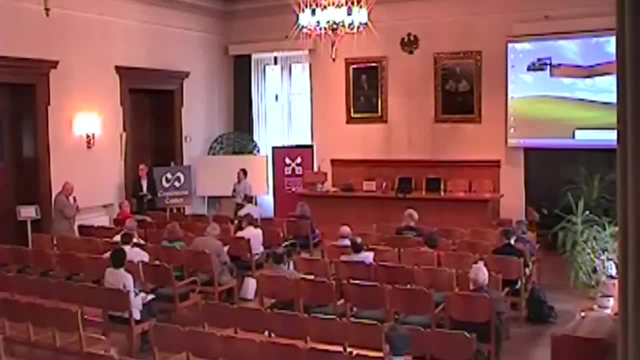 about truth Because it seems to me that, in order to operate, you should assume that arithmetic is omega consistent. In this case, Church's thesis is obviously false. You don't need intuition and so on, But without truth, because you have a list of arithmetical truths. 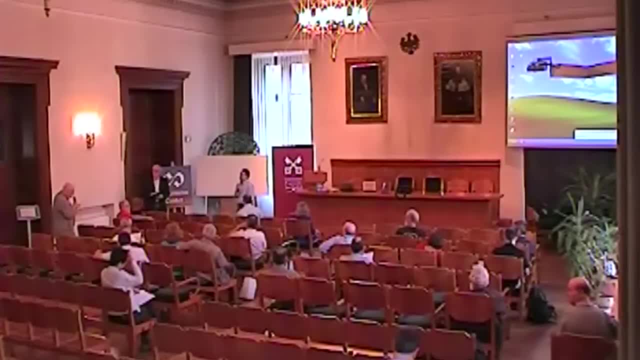 that is not axiomatizable, not intuitionistically given. So what is this? Because it seems to me that this assumption is classical. It is So. you prove in classical meta-theory that Church's thesis is under some assumptions false, But it doesn't solve any controversy. 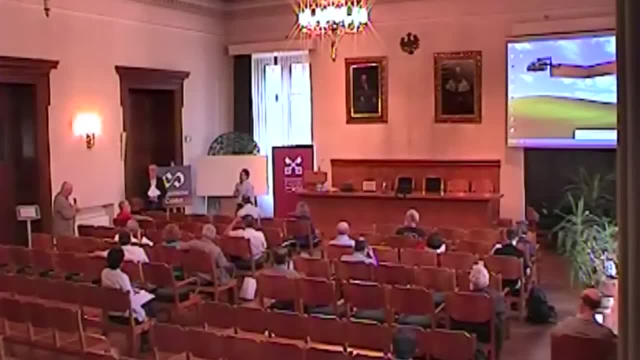 between realists and intuitionists, But I am indeed arguing that it does, And notice that these are all classical inferences. So all the inferences you so properly made from a conventional point of view are conventional, But there is a complete intuitionistic set theory. 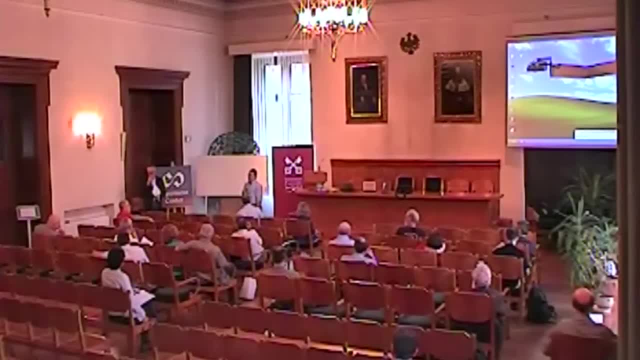 in metamathematics in which the inferences you mention fail. You can give a complete definition of truth a la Tarski, and yet Church's thesis is true, there And consistent. This is something that even a conventional mathematician could prove in the meta-theory. 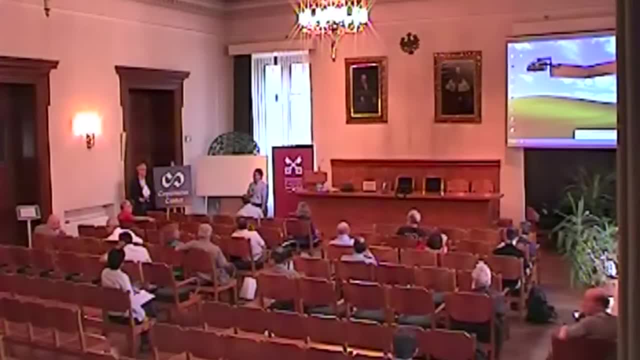 So if you are giving a cleanly realized ability interpretation to all of set theory, you can see that if the intuitionistic theory, including Church's thesis, the formal theory, derive a formal contradiction, then you would have to derive that formal contradiction in the conventional theory. The relative consistency proof goes through. 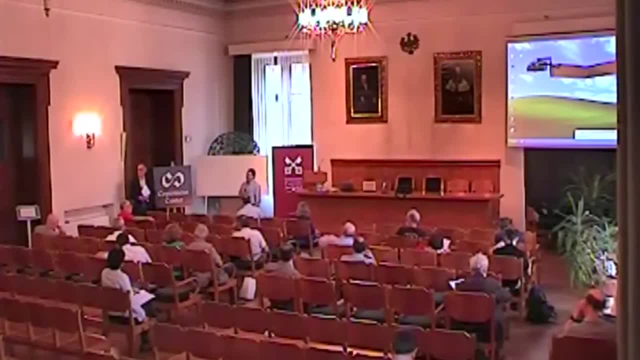 And this is all primitive recursive. I have two remarks. One concerns your result that every truth about intuitionistic nature holds also in the classical natural number theory. So if you think in what, second the so-called strong counter-examples to excluded middle rise in. 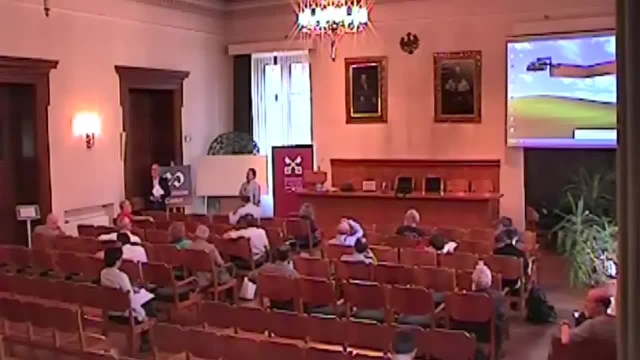 intuitionistic mathematics, it's always via continuity principle, Sometimes, Sometimes, So it's not always. No, No. Brouwer recognized three origins. First, as you know, the weak counter-examples- and these come from exploiting- they're not probative. 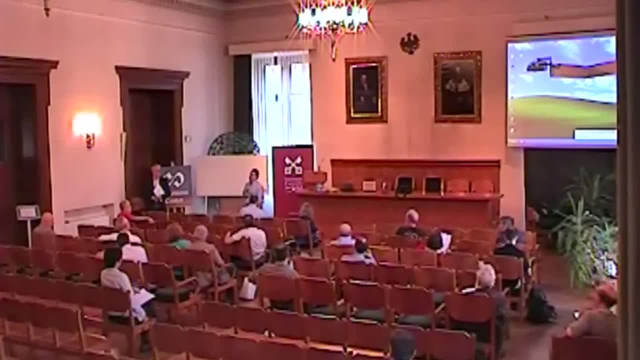 they come from exploiting so-called open arithmetic problems, Gold box theorem being one of them, Gold box conjecture. Secondly, from the continuity principle for numbers that Brouwer used Absolutely. Third, from Brouwer's creative subject plus continuity principles. 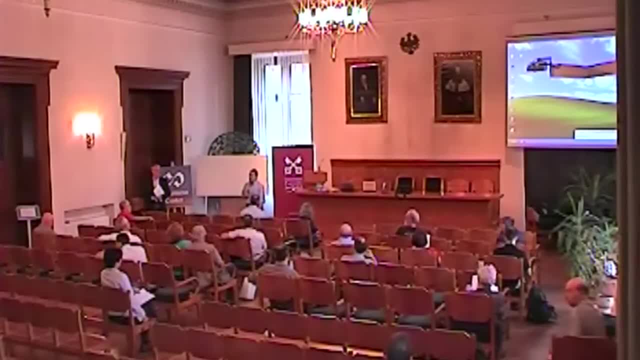 That's the third origin. But you need them because if you think carefully about it, especially in its form, in the Myhill-Kripke scheme form, it's classically correct. The theory of creative subject by itself is a classical theory. So in order to get the strong counter-examples, 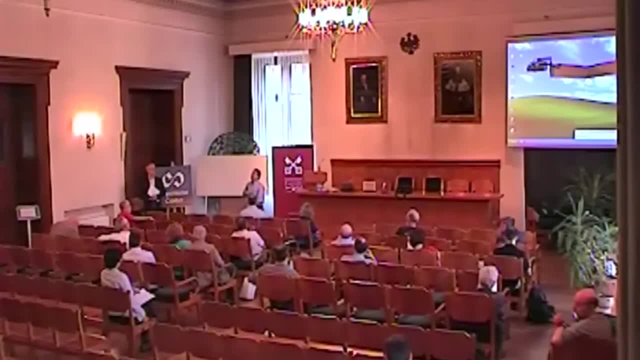 you must add something to that that's non-classical. The continuity principle would be one possibility. And then further, there are two other origins we have today and which Brouwer only pointed at these glancingly. Number one, what I call Church's Thesis. 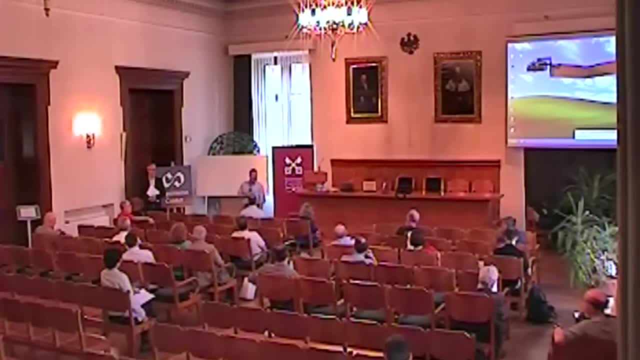 and number two, what I call the Uniformity Principle. Church's Thesis, as Kreisel pointed out, is a reduction principle for types over arithmetic, Reducing them all effectively to natural numbers. The Uniformity Principle then works at the higher order level. 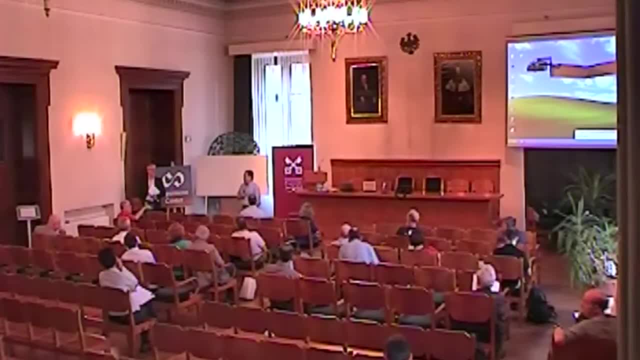 In governing arguments not relating functions on numbers to numbers, but relating subsets of the natural numbers to numbers, And from those various origins. strong counter-examples are all forthcoming. Okay, I want to proceed to my second comment, Please. I thought that you were somehow too fast. 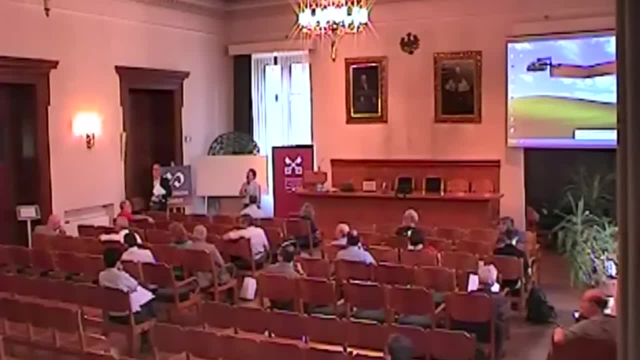 and quick with the negation. What's wrong, for instance, with Doug Pravitz's approach to intuitionism? That means, well, the difference lies in the elimination rule for negation. Okay, And then? well then the fact that 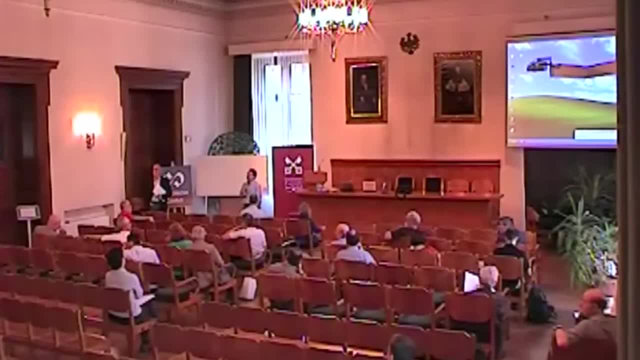 say things like versus law are the subject of controversy. that I explained by saying that basically you changed the concept of proof. So what's wrong with that approach? Doug Pravitz, you know Right, Notice what you've said there. I want to focus out. 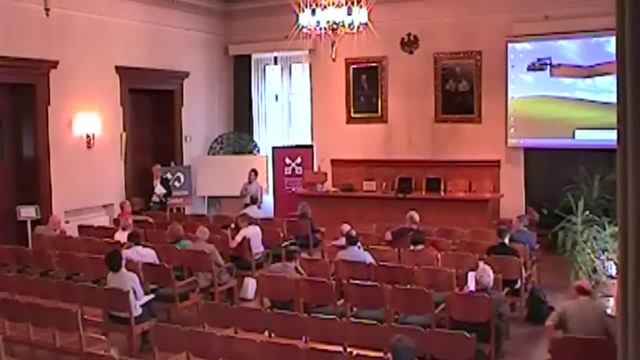 There's not one locus of change you're talking about. You're talking about changing negation and you're talking about changing the concept of proof. Yeah, because one influences the other. Yes, Insofar as logic alone, as we all know. 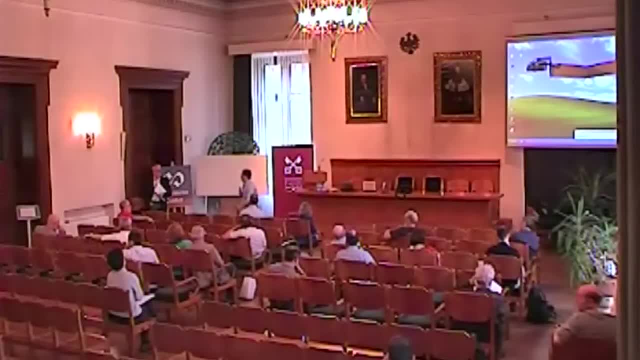 one can point to a variety, depending on the formulation, the formulation of the logic as to what the bone of contention you might well be. Often, negation is one of those, And there are other ways of formulating the differences of the logic. 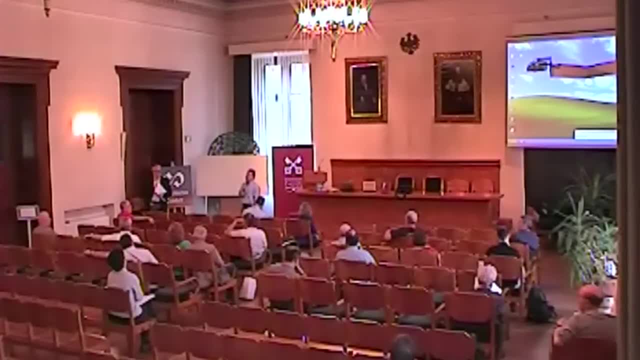 But then it's up to those who wish to show this to show that that difference about negation can be pushed into arithmetic and into higher type and into set theory. So you must continue to try to convince me that negation is the culprit all the way up the 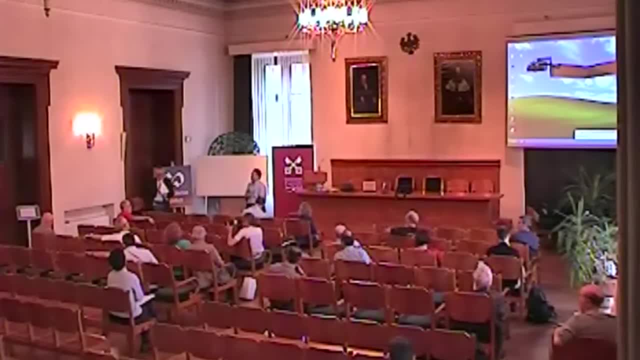 theory from the logic to the top. One more thing: The uniformity principle. it's the principle that tells you that if you've colored the power set of the natural numbers with numbers, that color has to be monochromatic. In other words, 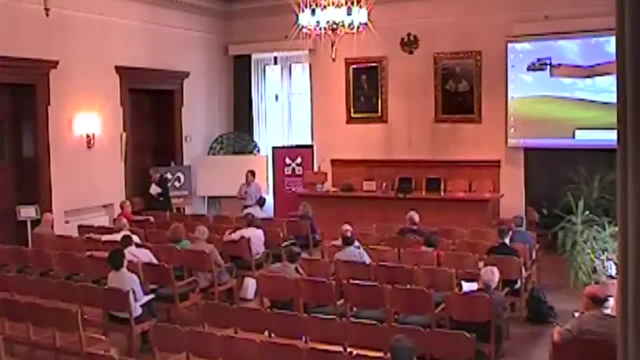 if you can assign a natural number to every set of natural numbers, then there must have been one natural number that you assigned to all of them. That principle does not involve negation in any way. So if I go over what you said by saying that negation is not the full story, 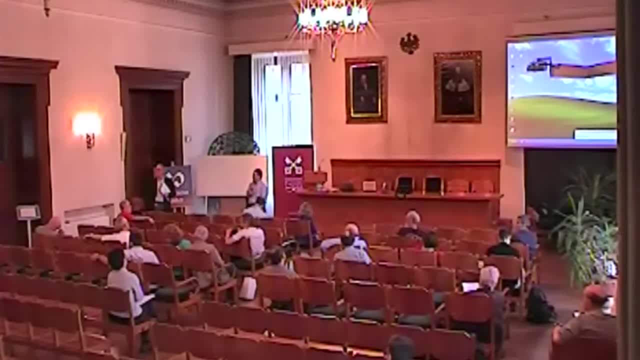 because of the continuity principle, bar induction, then do we agree? Yes, Thank you very much. Thank you very much for your comments. I would like to say that I like very much your two theses, which complete your work. Thank you for the conversation. 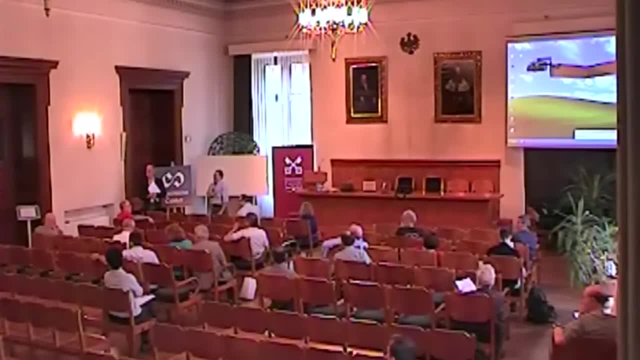 It's a fine question. I fully agree with them. But there is a part of your talk on which I have some unclear things, Maybe when you argue that negation, for instance, or quantifiers- intuitionistic quantifiers- cannot be compared with. 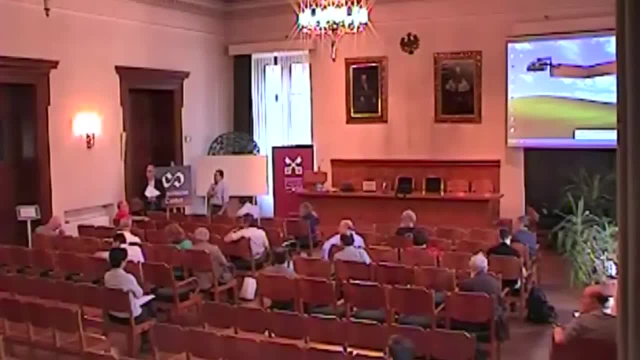 their classical counterparts, then it seems to me that you want to compare negation with negation, quantifier with quantifier, while in fact you have to compare the whole system, not just negation with negation, The rules of one logic with rules of another logic. 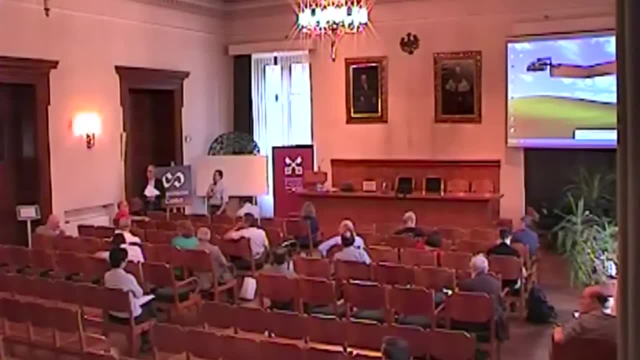 And the same is in the case of set theory. You cannot just compare one symbol for set theory with another symbol for set theory. So what I would like to say is something which is completely obvious, I believe, When you select different notations for intuitionistic logic. 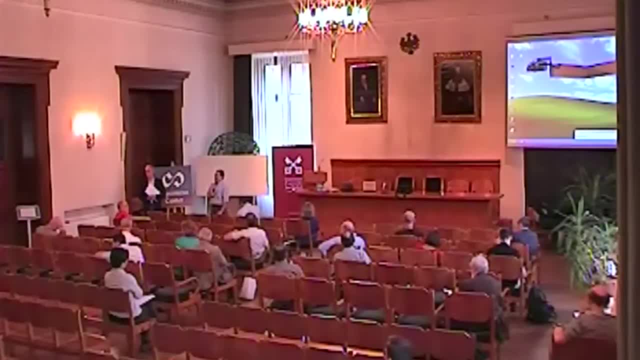 and classical logic for, say, set theory in which you have an axiom of choice that they contradict each other, then you can write them side by side And they will not contradict. The problem is with this bridging area because you have to compare. 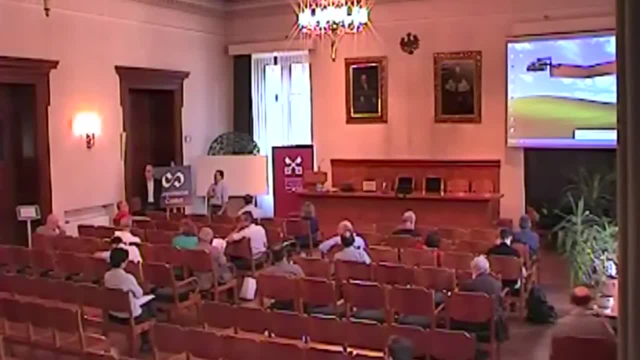 But from the point of view of classical mathematics you can compare classical mathematics with intuitionistic logic. You have some rules which will tell you what is true in intuitionistic, and such a comparison can be done also for set theories, of course. So this ignorabimus. 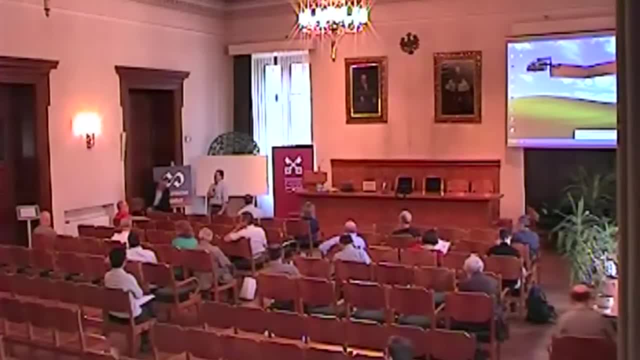 starts, in my opinion, somewhere in this area, when we ask how to compare these different ideas, And this doesn't prove that any of these ideas is better than another one, Though, if you take a look from the point of view of factual science. 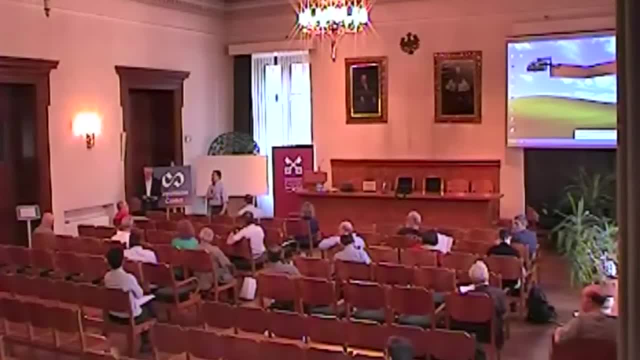 from those who are doing factual science, different from what I was doing. turning back to my talk- just only for a moment because I don't want to occupy time with my own ideas- then in some way, the classical mathematics is most natural. 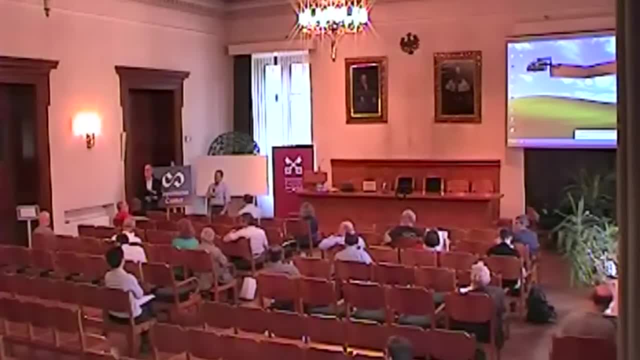 because it is strongest. This is what Popper argued. Take the strongest hypothesis at the beginning. Maybe that doesn't decide me between this determinacy and action of choice, but again action of choice seems to be stronger than determinacy. So maybe the breathing area. 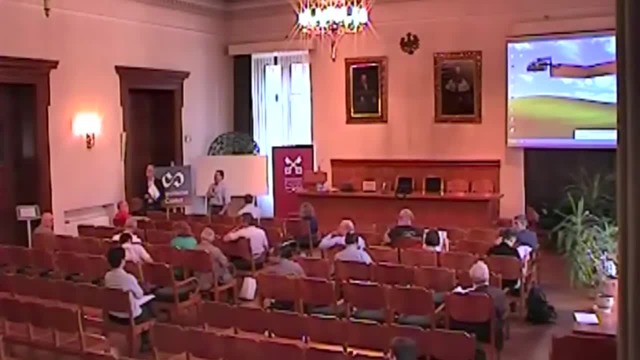 is impossible to find this breathing area. But anyway, if you look at the point of view of users of mathematics, maybe there is some choice between these two. Thank you. I do want to say that certainly the point of view being represented here is not one of holism. 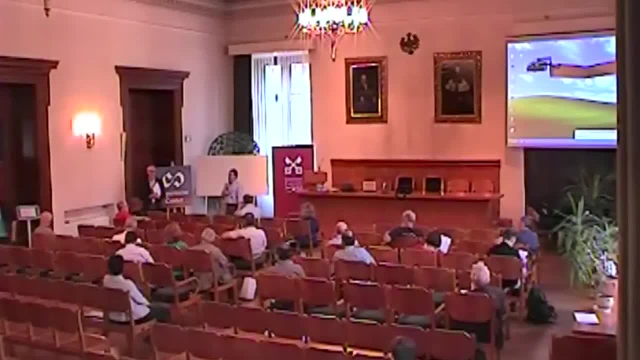 Indeed, I am not adopting the view myself that the only way to compare these two accounts is to compare them as formal theories, all together as units. So certainly that's a theme that's running through here. However, it does not seem to be a presupposition. 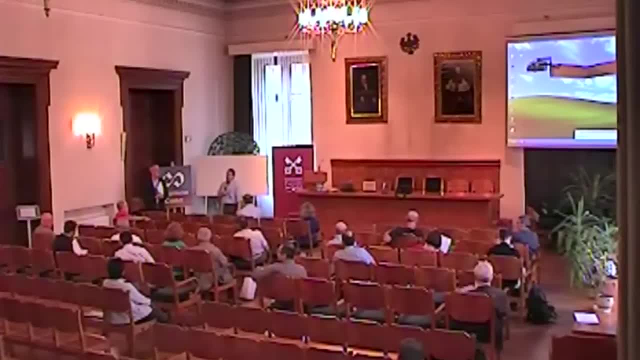 of the argument in question. Everybody in this room accepted when they read kindergarten. Everybody accepted the argument, So what's wrong with it now? Indeed, that is often said, that these theories must be compared holistically. I don't believe it, but it's often said. 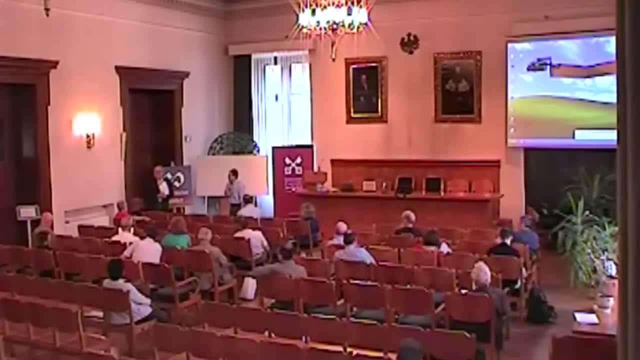 But where does that assumption come into the argument that I have broken something that is true and interesting? There are a couple of things I wanted to ask you about. You've convinced me, I think, that there can't be a single foundation, which I think is you're calling. 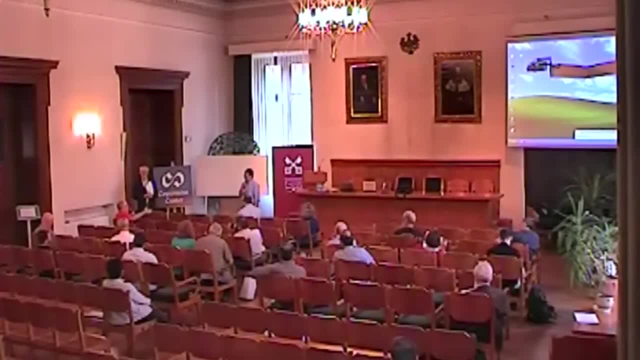 the realist assumption that there can't be a single ontological foundation for all of mathematics, And for the reason I think that you cited at the end, because there's no neutral place from which to assess it, But I'm claiming it's certainly. 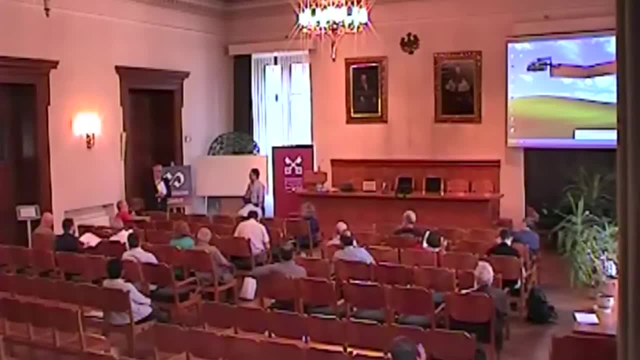 highly suggested by the argument. How are we going to address the problem? if we don't like the contradiction, Well then it would have to be to give up the idea that there's a single foundation. Now, of course, what you want to say. 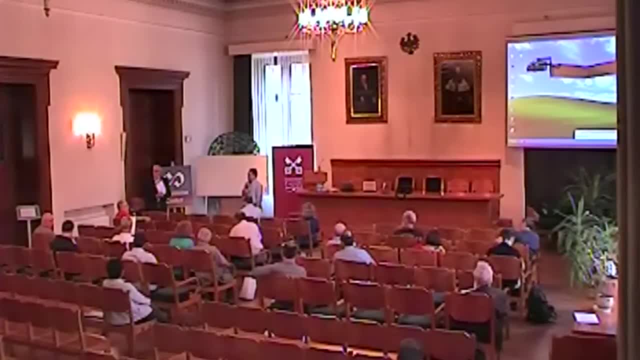 after that is, people are going to disagree about that. The thing I wanted to ask you about, though, is the thing you noted at the beginning. It's a theme you've been emphasizing for a number of years now, With that little show you did. 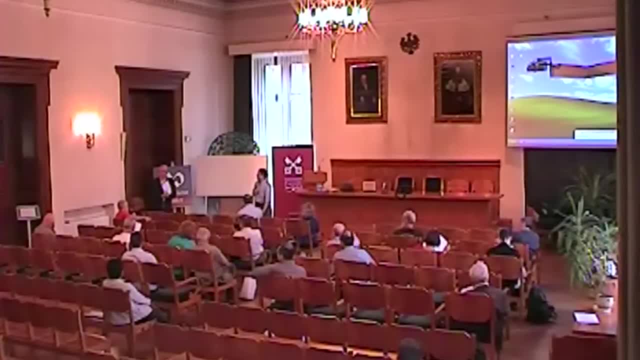 in the beginning A little dialogue waiting for Bob. Now you might not think much of it, but there's a big industry now in philosophy of language of trying to figure out generally when words have the same content and when they don't with other. apparently. 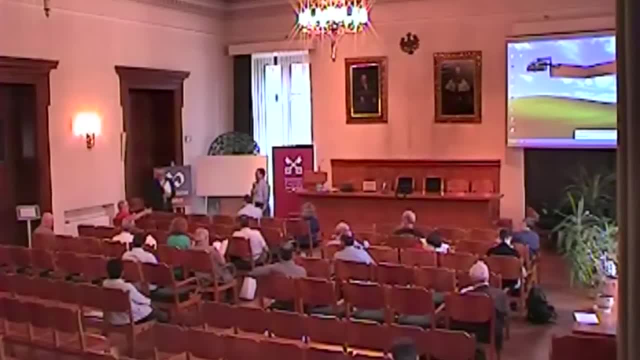 context-sensitive terms, Words like to the left, to the right, enemy, predicates of personal taste. And then there are sort of little tests, But there are tests that everybody is trying to develop for when you have the same content and when differ. 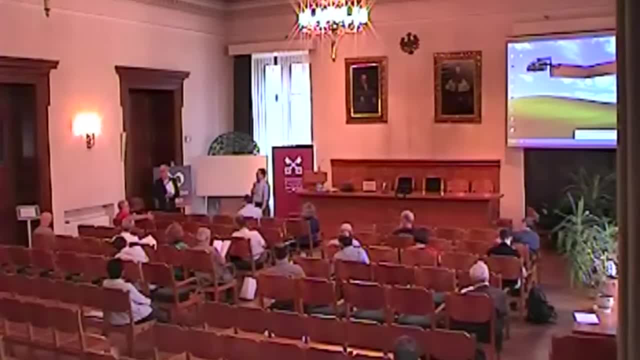 Have you thought that any of that might help to adjudicate the question that we're interested in? Is the meaning the same? That is an interesting thought and I'd like to pursue it, and I don't know the answer to that question. I thank you for the idea. 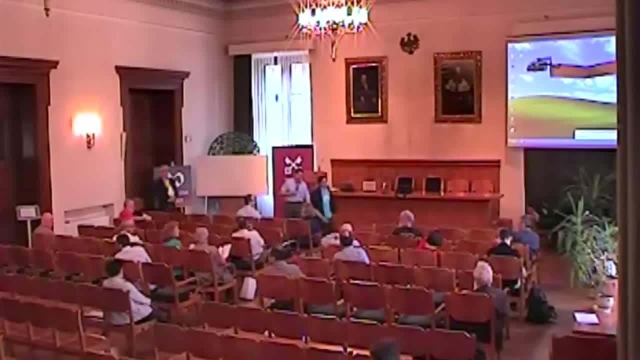 After the talk I'll get started. Thanks, Stuart. Look, I'm a little bit slow person, so it was very. I couldn't really follow all the proofs and the details to check whether it's correct or not correct. So what I say is: 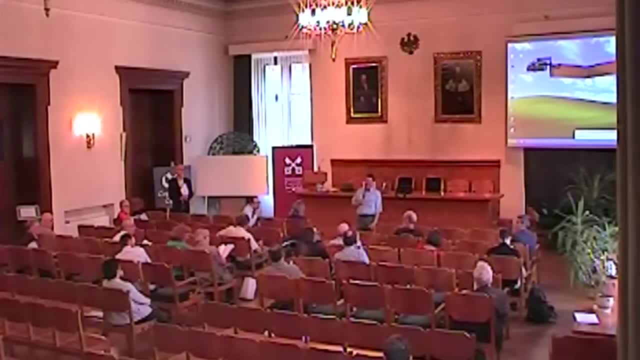 Superficial understanding. So, if I understand correctly, you say that you derive contradiction from some assumptions and you blame, And the conclusion is that something goes wrong under realism or no single foundation of something. Well, notice that these were not conclusions of the central argument. 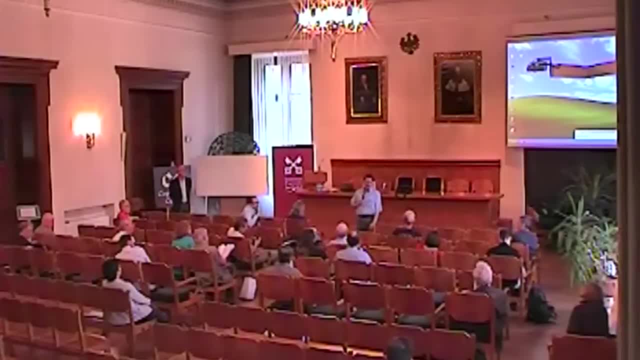 The conclusion of the central argument is this: If you accept a very watered down form of realism, that is, that mathematical theorems have their power over us in virtue of there being true reports upon the behavior of mathematical things and the components of those things, 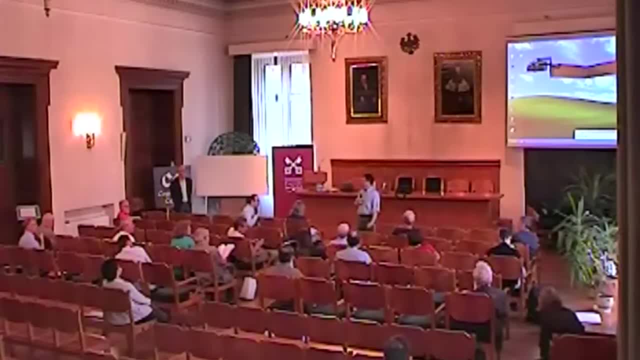 if you accept that assumption, then in simple mathematics, simply pointing out that there is a second-order classical arithmetic, that there is a second-order intuitionistic arithmetic, they're both consistent From those assumptions and Datikin's argument that all models of second-order arithmetic. 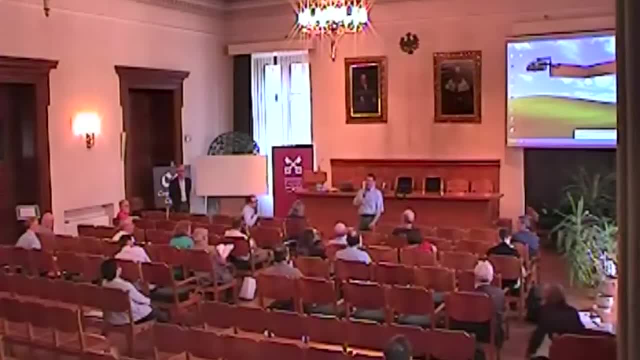 are isomorphic, a contradiction follows. That's the argument. Now, from that these other claims do not follow strictly, but I think they are suggested. However, the proof, the detail of the proofs. sorry for being so old-fashioned. 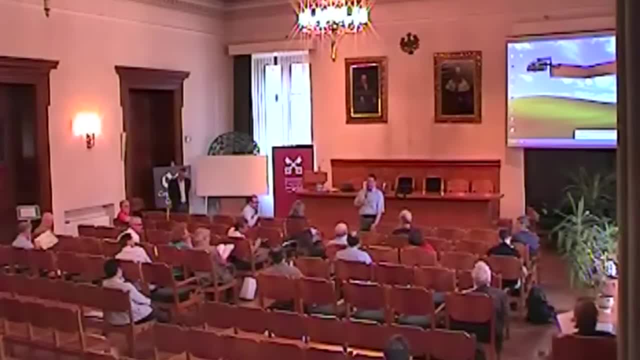 but in order to really understand, to find out what is, if there is a proof of contradiction, what is the? who is to be blamed for the contradiction? because usually there are, in any proof of this, several assumptions used. Yes, 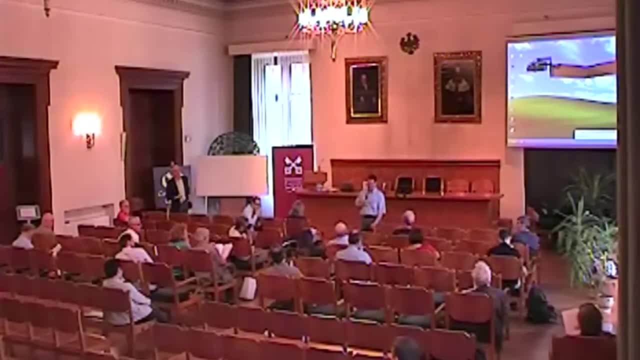 And I, to really believe, should know what exactly are the assumptions, what is the language, how to formalize it. sorry, if you're switching: from one place you're talking intuitionistically, another place you're talking classically, and after I see. 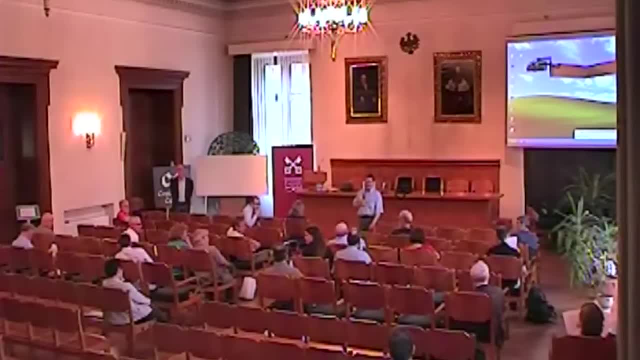 see how to formalize- not really fully formalize, but see how to formalize it. see exactly what the assumptions. I would tell what is responsible. But something about my impression. first of all, it's not true that you have not used 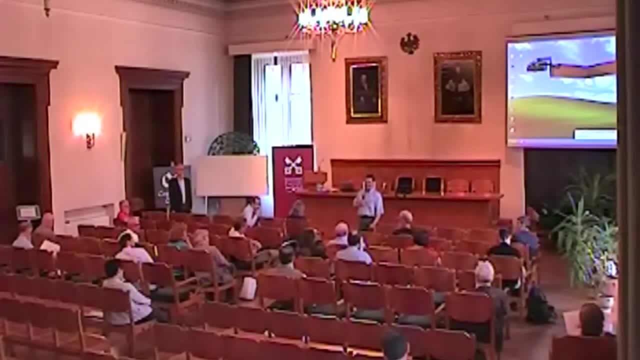 any foundational issue. I've looked very carefully. you use the term functions, components, class, and so all of them come from one foundational: no categories, no structure. but in order to understand what you have said, you have to understand this basic notion. 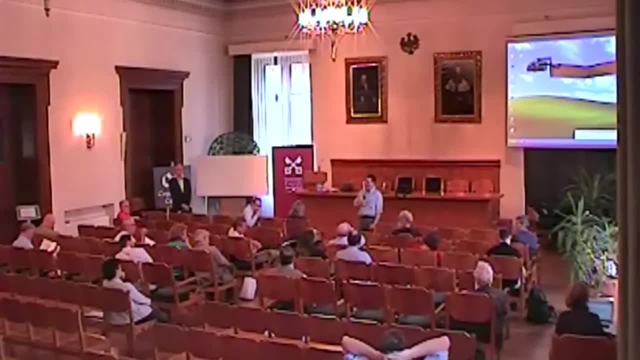 of the foundation user foundational things without it. at least, we need to prove that every every. to me, it seems that you use circular because there exists some function that give this and this, and this is all what you have to prove exactly. 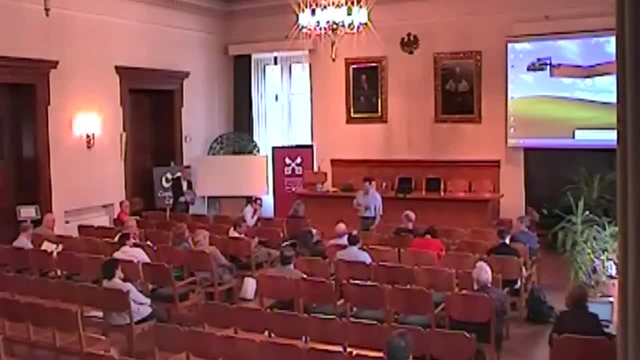 So my impression again, because it's a short time and one cannot follow this in short time- my impression was that sometimes you're using terms, assumptions that are more or less equivalent to what is to be proved in other place. 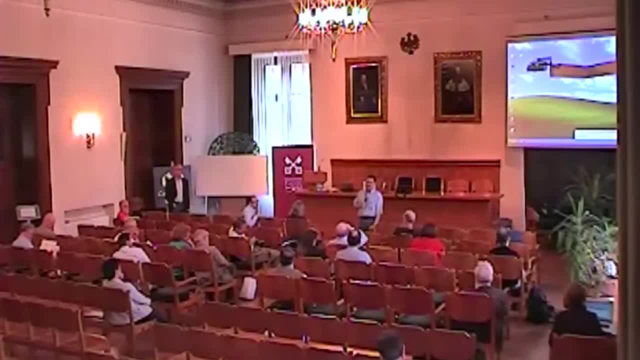 you pretend to talk about what, but really you know exactly what are the what nots. Notice that I have not asserted that I would not be using foundational notions at all. you're absolutely right. I'm employing standard foundational notions like set, function, complement. 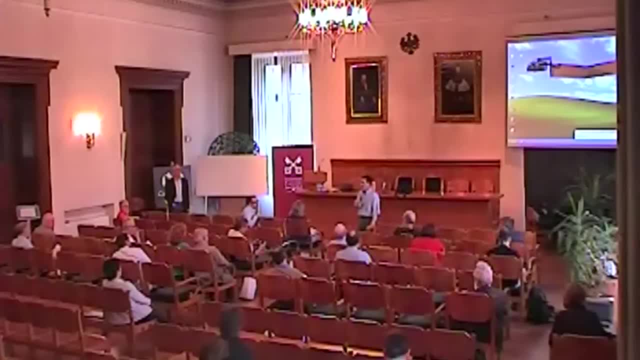 equivalence relation, equivalence class. there's no question, I could not get started without those and their basic properties. What I do maintain is that none of those basic properties that I listed, you listed and used are controversial between the intuitionist and the classical mathematician. 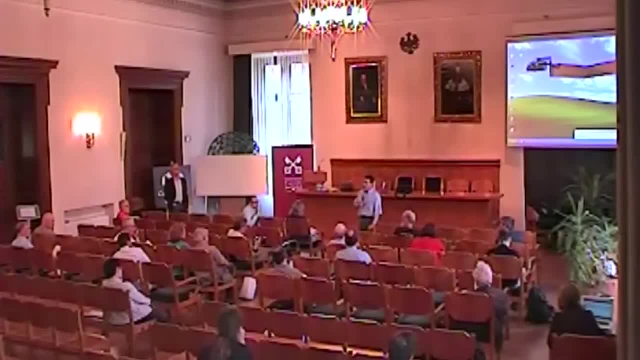 they are common coin to both. So I have not used any foundational notion that could be rejected by either party to the particular dispute, But the proof of the use of fundamental functions is clear, Right, But if that, I give the same answer that I gave before. 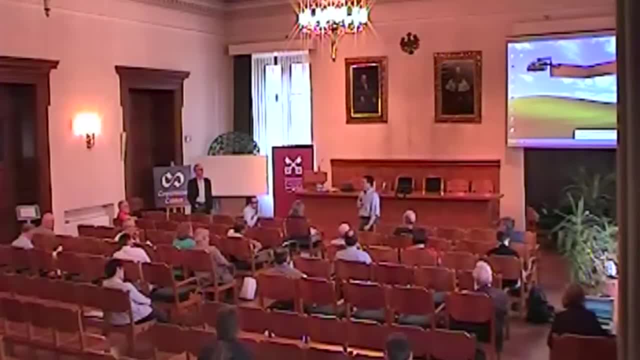 If there is a difference in the notion of function, show me where that difference is. Well, hold on a second. I love this. I love this guy. We've been arguing like this for how many years? 25?, 26?, I hate to say it. 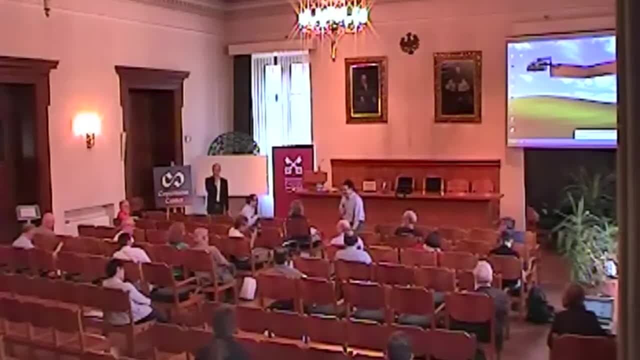 But let's have fun doing it, though, right? I think we may be out of time, I guess. Well then, just very quickly, What's the role of Church's thesis in the deduction of the contradiction? Well, it is not so. 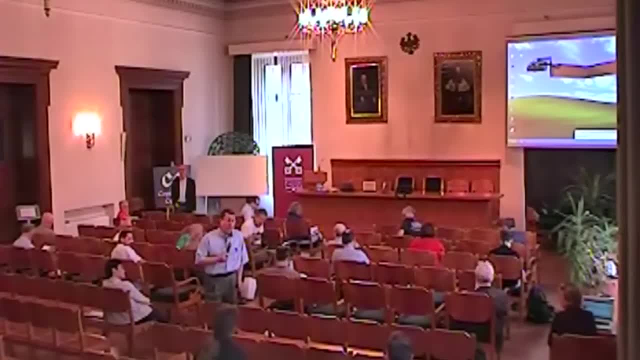 It has a large role to play in intuitionistic mathematics as a whole, as Kreisel liked to point out Here. it's simply an example of a statement on which the classical mathematician, classical arithmetician and the intuitionist will disagree. 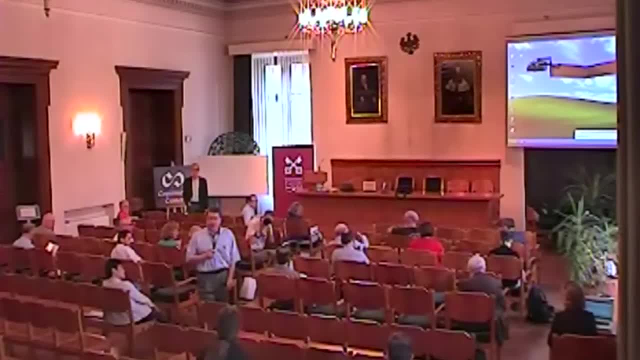 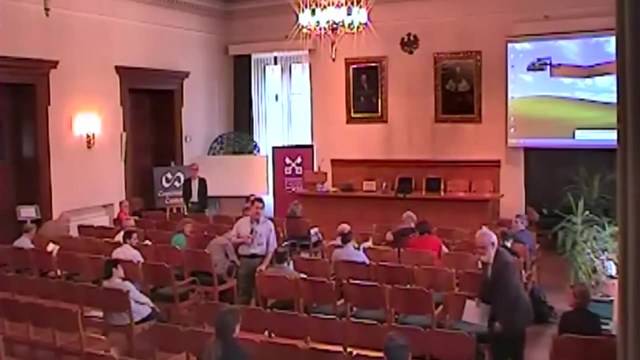 One believes that it is absolutely false in the arithmetic classically. The other believes it is absolutely true in the arithmetic. I could have chosen any number of different statements. I chose Church's thesis here for the obvious reasons. I should also very quickly point out: 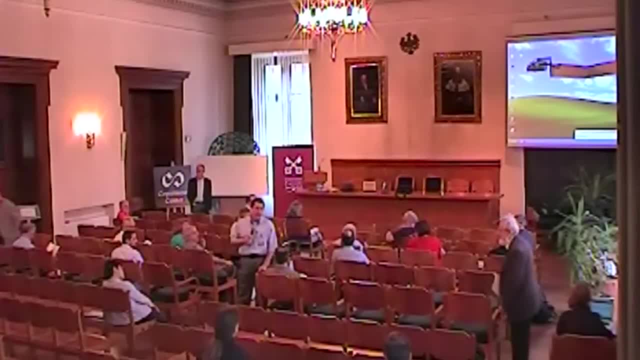 Church's thesis has uses in intuitionistic mathematics. One of the most prominent is showing that there's at most one model up to isomorphism of first order arithmetic. That's one of the uses here, So its use as a reduction principle is powerful. 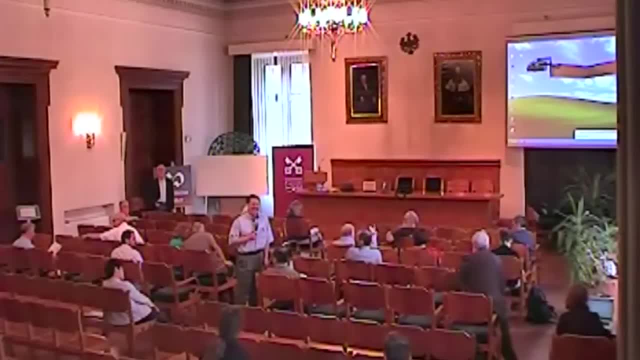 But it doesn't have any crucial role in the general pattern of your argument, right, It does not? I could have chosen any statement of arithmetic on which the two principles differ. Is there any commonality among the principles that you would choose there? 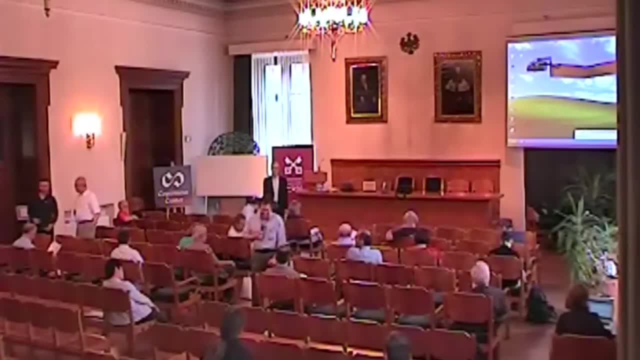 I mean in this particular instance, it so turns out that those tempted to hold it's false, Like everybody in the room but me. Well, I don't know, But there's certain relationships between that position and the classical versus intuitionist. There are. 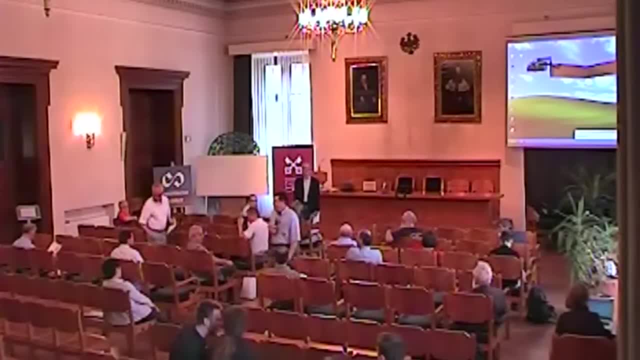 They need to be better investigated, but there are definitely relations between them, Thank you. Thank you, Wilfred, Thank you, ladies and gentlemen.